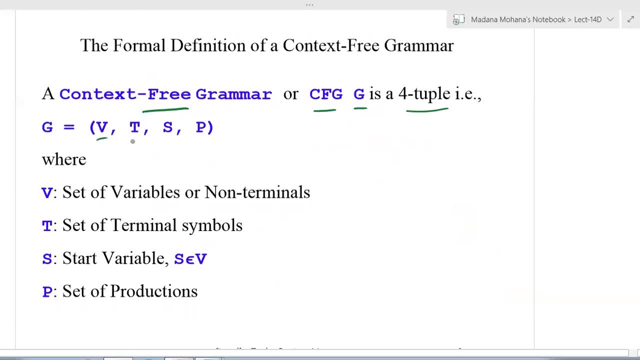 variable that is defined by a combination of VTSP, therefore G equal to VTSP. Where V is a set of variables or non-terminals, P is a set of terminal symbols, S is a start variable. where S belongs to V, Then P sets a set of production. Now the productions are of the form. 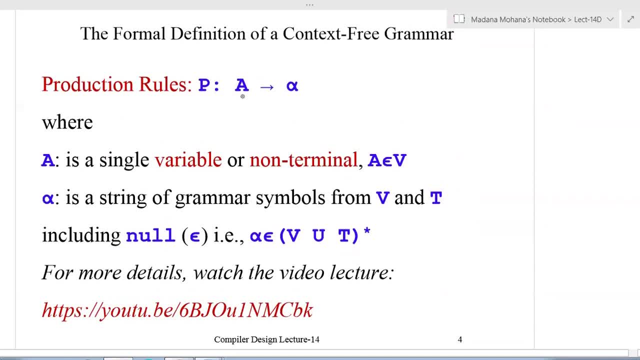 the production rules. P is a mapping from A to R, alpha, where capital A is a single variable or non-terminal. where A belongs to V, Then alpha is a string of grammar symbols from variables and terminals, including null, that is epsilon. So then alpha is formally denoted as alpha belongs to V. union T, whole closure. 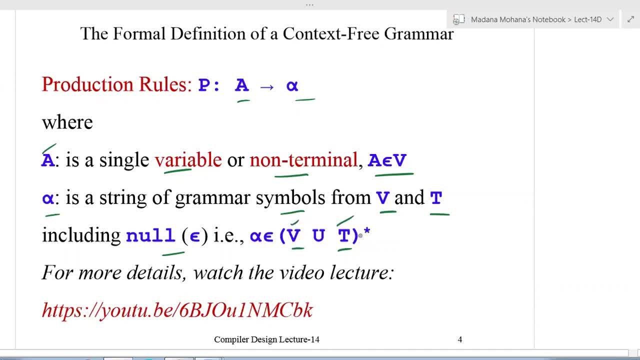 So here V means variables, T means terminals, closure means, which includes null also. Then, by repeating VT, ones are several times. So these are all string of variables and terminals, including null. Then the full lecture regarding this context-free grammar, watch the following: 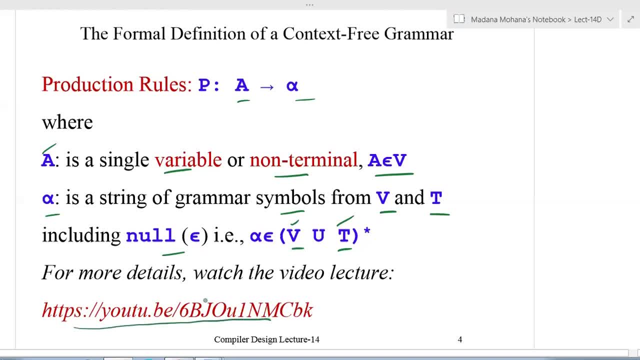 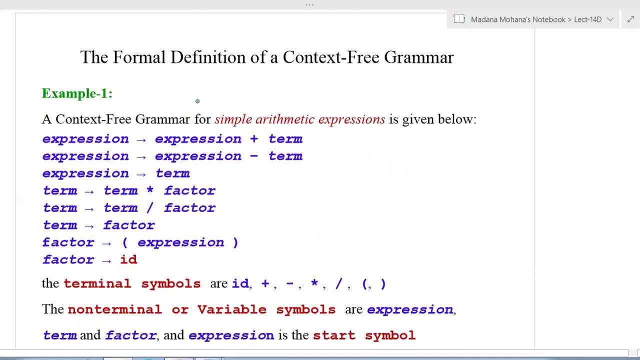 video lecture where we discussed informal language and automata theory. Now let us see some examples here. First, A context-free grammar for simple arithmetic expression is given below: Expression equal to expression plus term. Expression equal to expression minus term. Expression equal to term, Then term. equal to term into factor, Then term equal to term by factor, Then term. 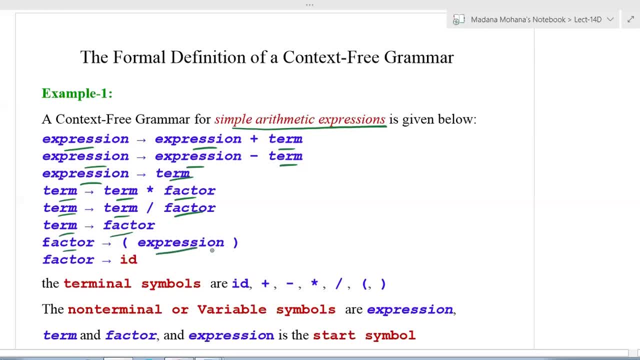 equal to factor, Then factor equal to expression within parentheses, Then factor equal to id, which stands for identify. In this grammar you can observe that terminal symbols are non-terminals, Then the non-terminals are variable symbols, or So left hand side each. 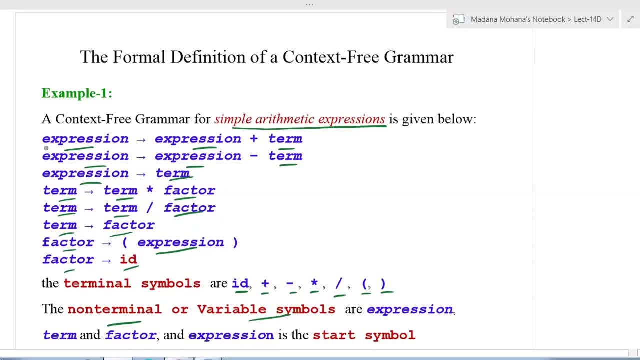 and every production starting with some variable. Those are all the variables. Then same names occur in the right hand side also. Those are all called as variables. Now in this grammar the variables are expression, then term factor, and expression is the start. 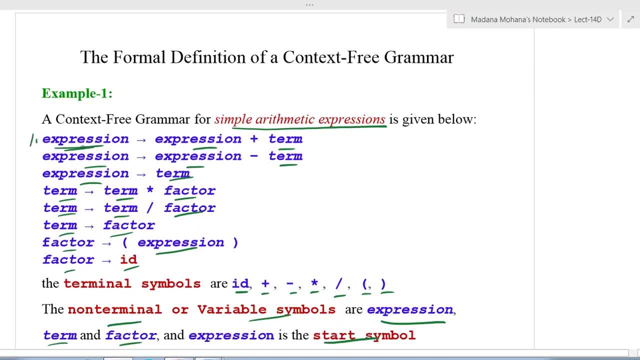 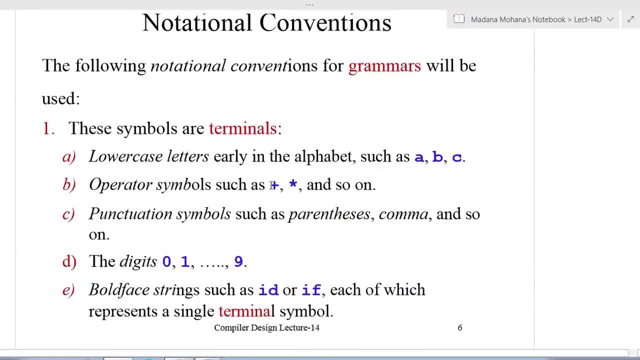 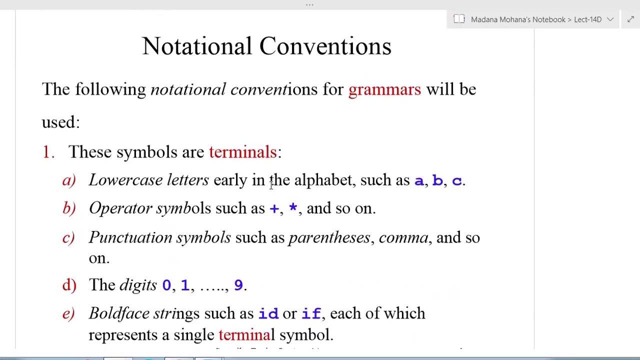 start symbol, Because the first production, left hand side, starting with expression, therefore expression is the start symbol. Now let us come to notational conventions. So what type of notations will use for representation of variables and terminals in the grammar? The following notational conventions for grammars: 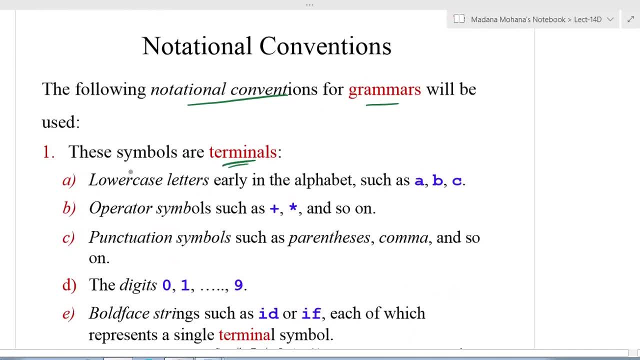 will be used. First one terminals. The following symbols are used for representing terminals, That is capital T in the grammar. All lowercase letters only in the alphabet, such as a, b, c and so on, are terminals. Then operator symbols such as plus, into and so on. all are used for. 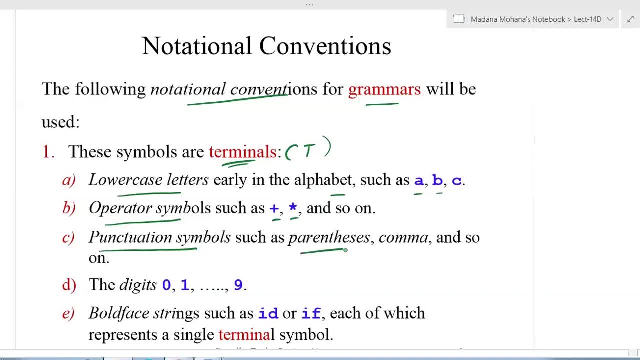 representing terminals. Then punctuation symbols such as parentheses, comma and so on are used for denoting terminals. Then the digits 0 to 9 are used to denote terminals. Then bold face strings such as id identify some keyword, if each of which represents a single terminal. 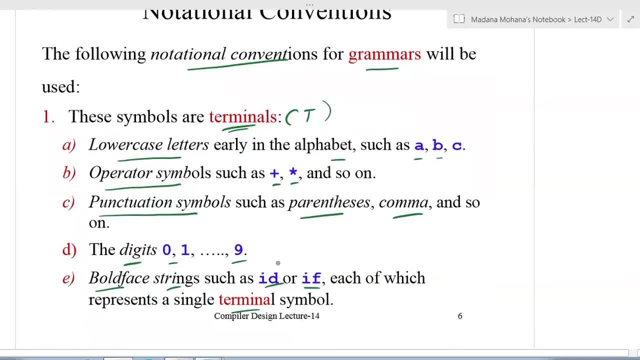 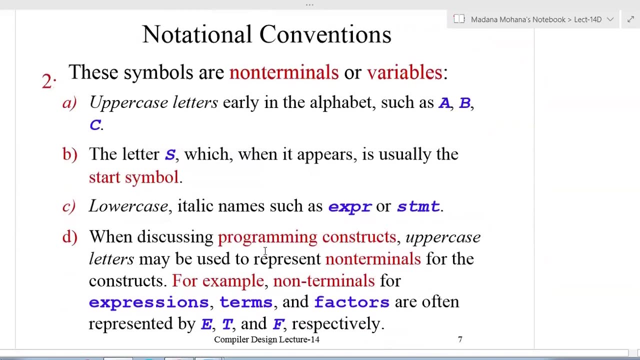 symbol. Don't consider it as i and d separate, i and f separate. So whenever we are representing with bold placements with bold, so these two symbols can be treated as a single terminal symbol. Then those are all the user notations for representing terminals, Then for the other, 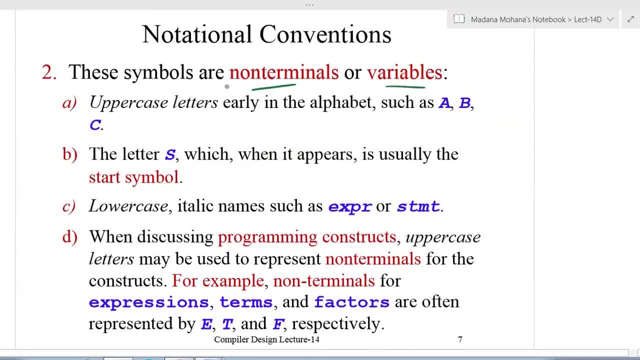 notations they are used for representing terminals, Then for the other notations they are used for representing non-terminals or variables. So these symbols- that means the following- are used for denoting non-terminals or variables. Uppercase letters only in the. 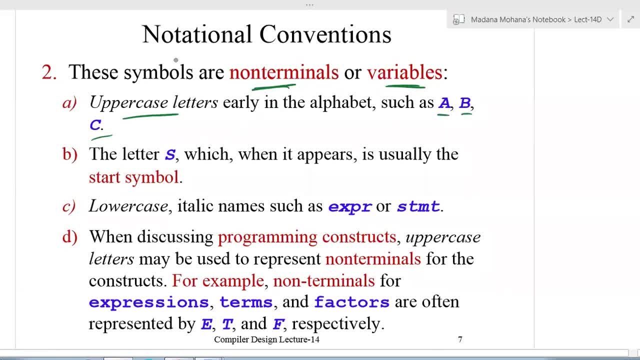 alphabet: capital A, capital B, capital C and so on are used for representing non-terminals or variables. Then the letter capital S, which when it appears is usually the start symbol, Then lowercase. some italic names, such as expr or statement, are also used for denoting. 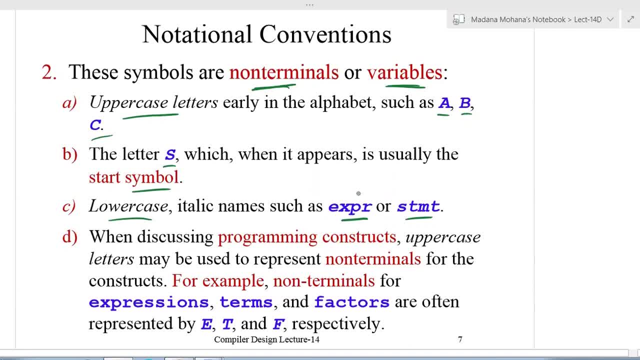 non-terminals or variables. In our previous example we have expr, stmt, so with lowercase italic names. So denotes the non-terminals or variables. Then when discussing programming language constructs, uppercase letters may be used to represent non-terminals for constructs. 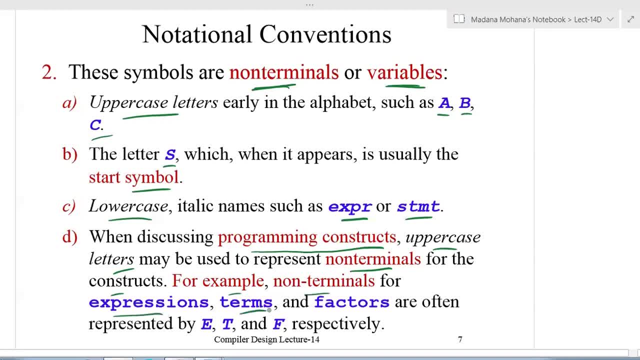 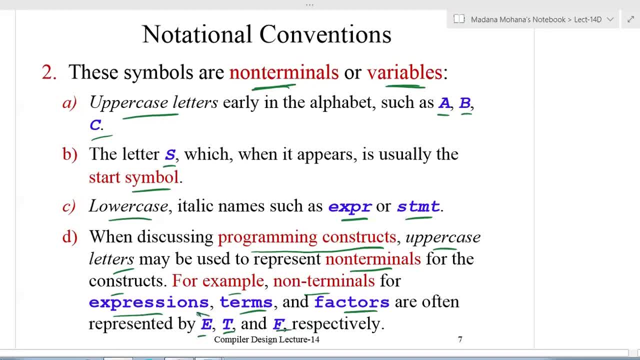 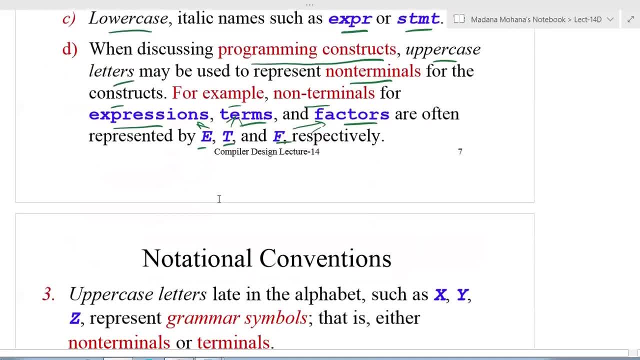 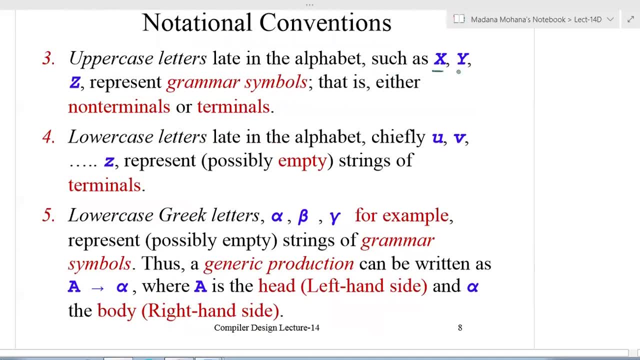 use it for denoting non-terminals or variables. Then uppercase letters late in the alphabet, such as X, Y, Z, represent grammar symbols. So then these are either type individually built loopholes, Lex and le are their grouped individually, So we can use letters based interchangeably and use the alphabets to put letters. 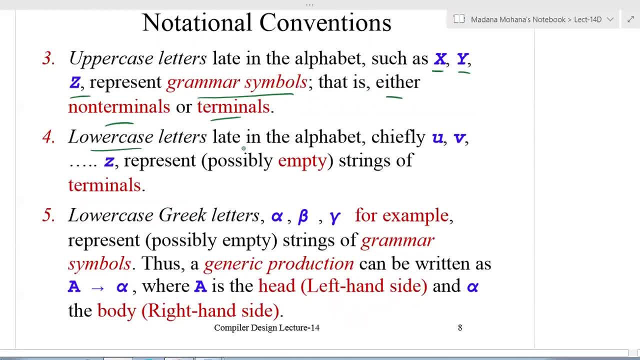 non-terminals are terminals. then lowercase letters late in the alphabet- that means letter symbols like u, v, w, x, y, z- represent possibly empty, including empty. so which represents strings of terminals, because these are all lowercase letters. then lowercase greek letters, also- alpha, beta, gamma, for example- represent possibly including empty string of grammar symbols, thus a generic. 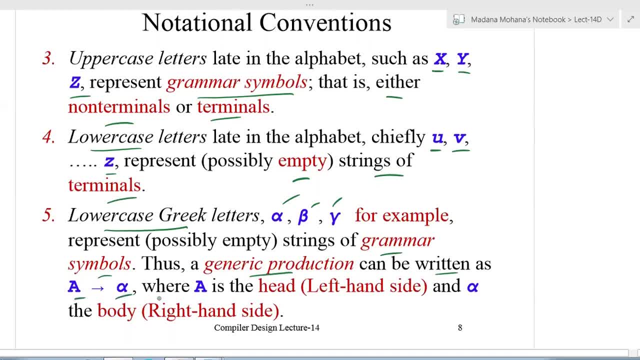 production can be written as a derives alpha, where capital a is the head which can be placed in the left hand side and alpha is the body which can be placed in the right hand side. suppose for a program, so header, then the definition of that header, so like here, a. 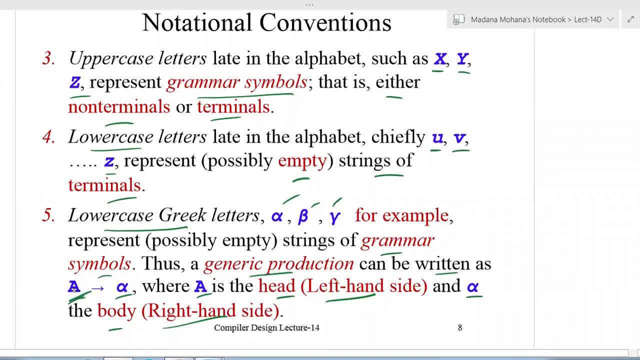 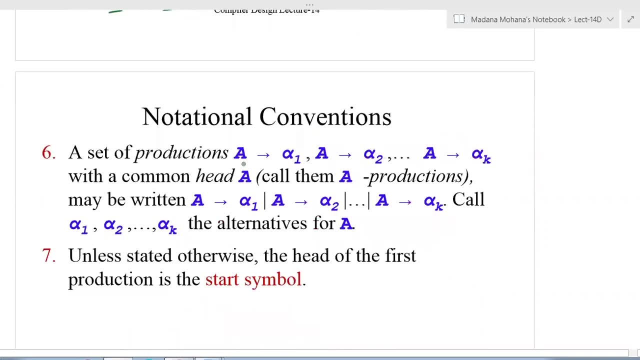 derives alpha a is called as header, in the left hand side, which is called as a variable, then alpha in the right hand side, which is called as the body of that production, where alpha is string of variable or terminals, possibly null. also then a set of productions like a derives alpha one or 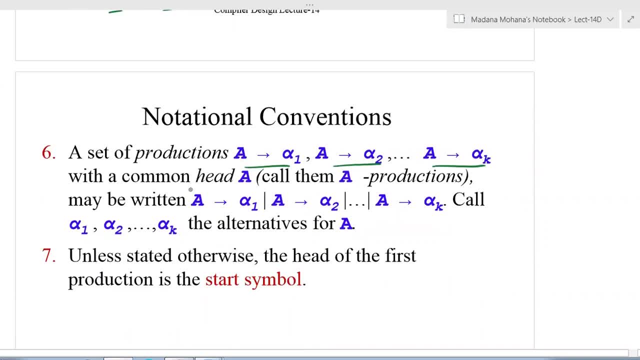 a derives alpha two and so on. a derives alpha k with a common head, a left hand side single variable is there. call them a productions. now, this is all called as a productions because starting with the left hand side, same head, a, and may be written as: by combining all these, a derives alpha one, or by separating with or multiple. 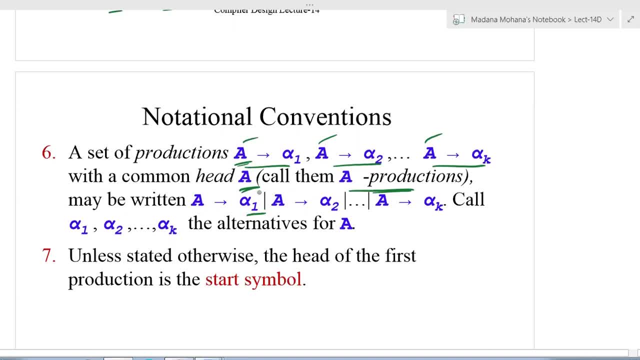 productions. you can combine a derives alpha one, so here this is not required, or alpha two and so on, or alpha k, so call alpha one, alpha two and so on. alpha k are the alternatives for a. that means, here this can be written as a derives alpha one or alpha two and so on. alpha k because 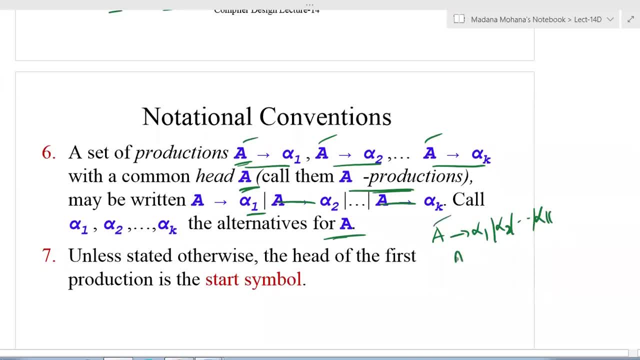 all are starting with a. so if you can split again, this will become a derives alpha one, then a derives alpha two, and so on a derives alpha k. so all these are starting with common head, a. therefore, this can be combined by using r, then another one, unless stated otherwise. 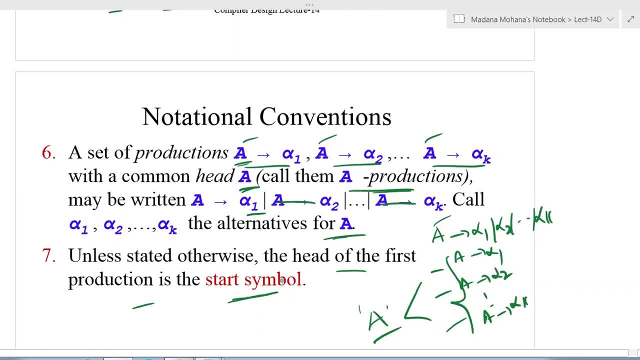 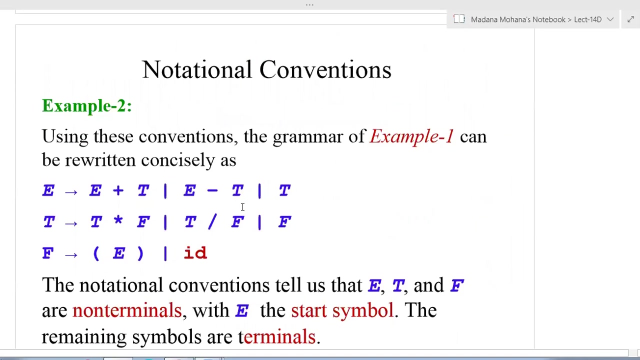 the head of the first production is the start symbol. suppose in any grammar the start symbol is not defined, then you can identify by seeing the starting production, the first production, left hand side, whatever the variable or non-terminal that can be treated as the starting variable of the given grammar. now let us continue with other examples. example two: so using these, 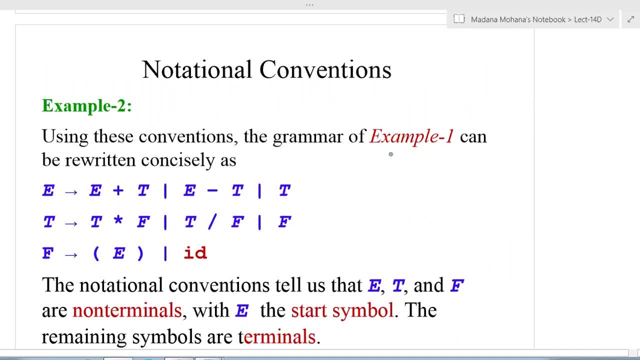 conventions? what are the notations we mentioned? the grammar is not defined in any grammar. if we have infinite words for notations and letters, zml, all should be defined with z terminals. therefore, why don't we try another step? for example, we have an associated, very basic, simple. 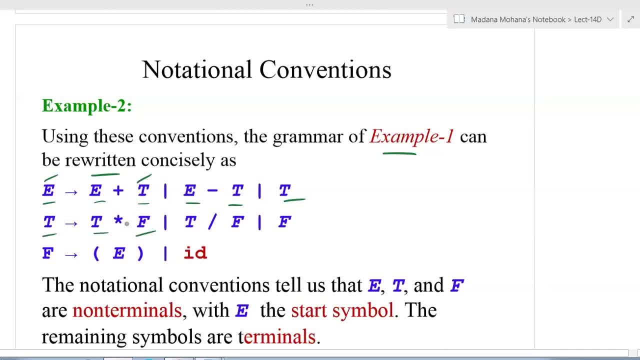 proof of the example one can be rereaded, and politely as that, both grammar, these expression term by factor or factor. so where f is factor, now factor is defined as e, within parentheses then, or identified. the notational conventions tell us that e, t, f are non-terminals with e. 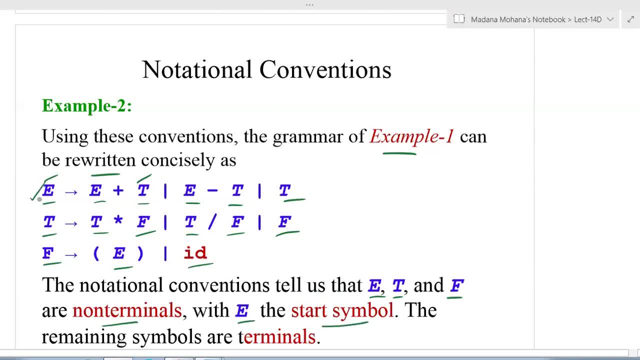 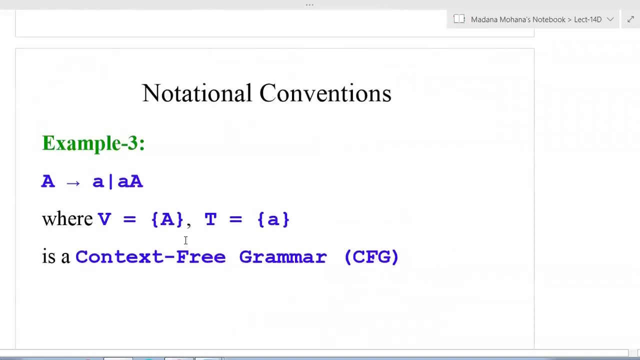 is the start symbol. the first production starting production in the left hand side, e is the is the start symbol. the remaining symbols are terminals, like all the operators plus, minus into divide, then parentheses, then id. these are all terminals. now another example. let us see variable a derives terminal a, or terminal a or variable a. here the variables are only one. 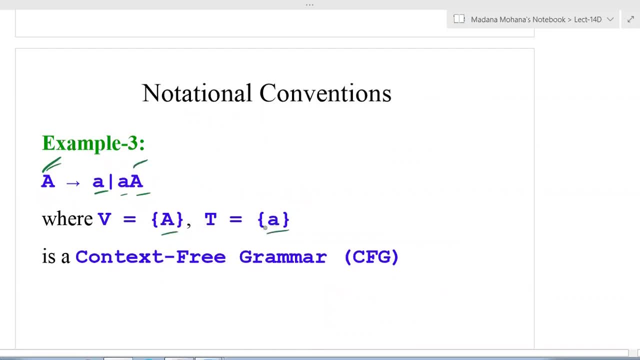 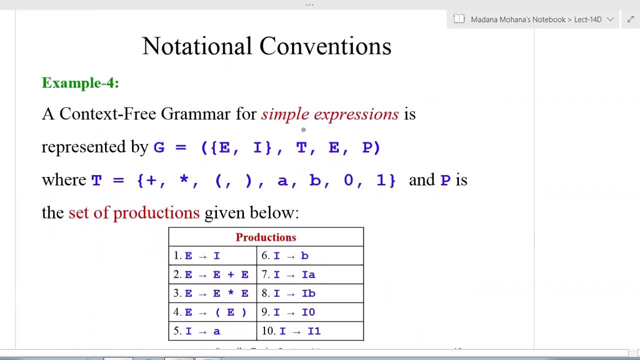 variable. we have capital a, then terminals are only one terminal, small a. this is also a context free grammar, so like that, different examples are given here. another grammar for simple expression represented with t equal to e comma i: this is nothing but v. you then t, this is nothing but yes. then p production, where t plus into left parentheses, right parentheses. 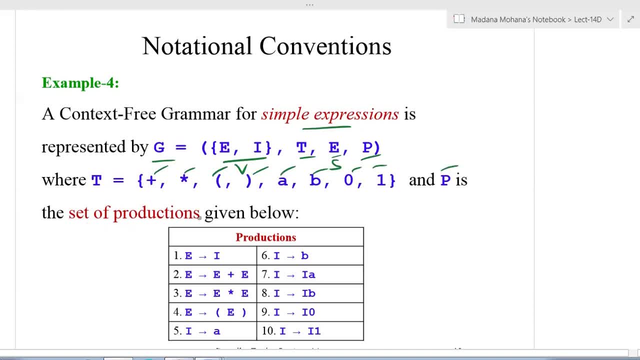 small: a small b, 0, 1 and p is the set of productions given below. e derives i, a derives e plus e. e derives e into e. a derives e within parentheses e, then i derives a. i derives b. i derives ia, then i derives ib. i derives i 0, i derives i 1. this is another example of context, free grammar, so like: 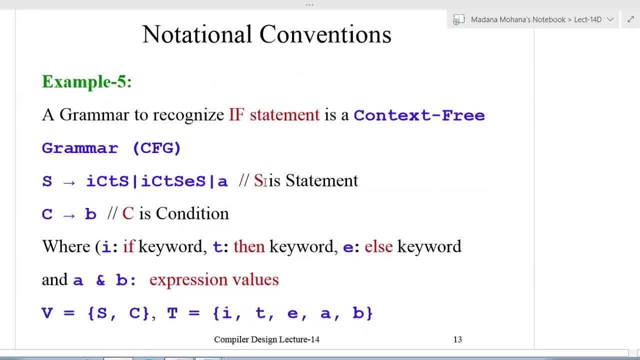 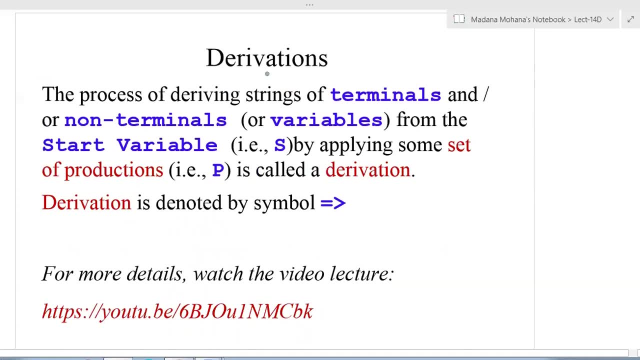 that that any example. by using the above notations, we can define the context in grammar. now let us move to the concept of derivatives. so derivation is nothing but the process of deriving strings of terminals under non-terminals. that means our variables from the start. variable, that is capital. yes, by applying some set of productions. that is smiling. 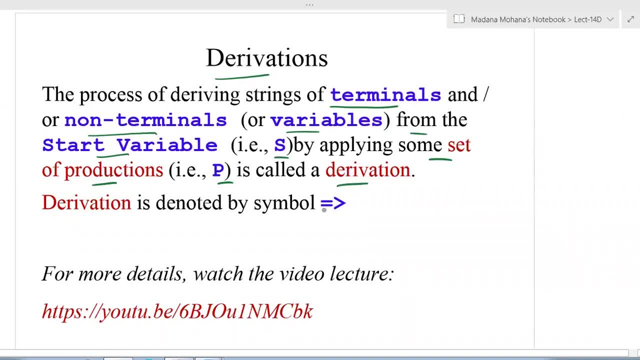 t is called a derivation. derivation is denoted by the unit쉬 wowgi. theres a lot of great evidence to show that the toxic plus is obsessed with observing a situation called pie in which use an ax. these operations are to predict how the workspace concept or 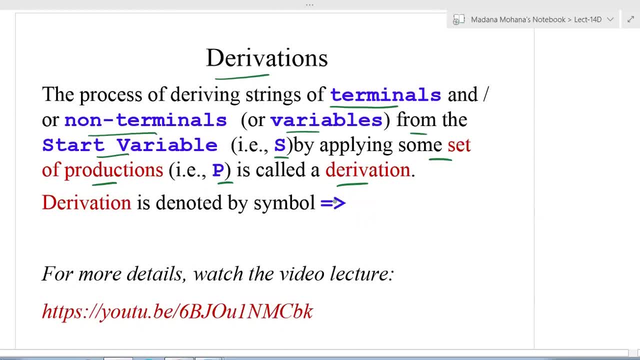 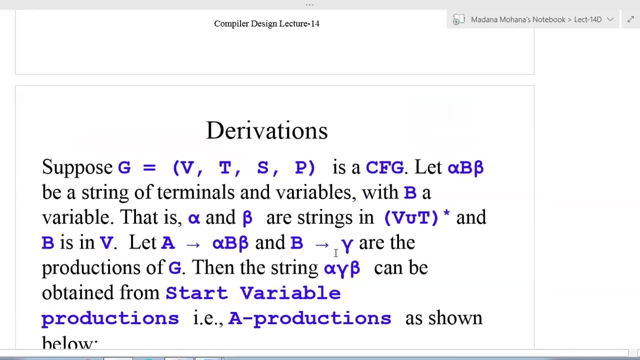 unidirectional double arrow, unidirectional double line arrow. then for the concept of derivation, where we studied in formal language and automata theory, you can watch the following lecture for the concept of derivation. so now, formally, how to define this derivation. suppose g equal to vts. 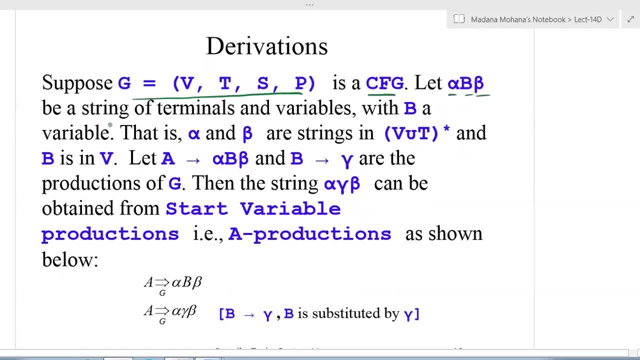 v is a context diagrammer, then let alpha b, beta be a string of terminals and variables where capital b is a variable, that is, alpha and beta are strings in v- unity, whole closer- and b, capital b is in variable v. now let the productions for capital a and capital b a derives alpha b, beta. 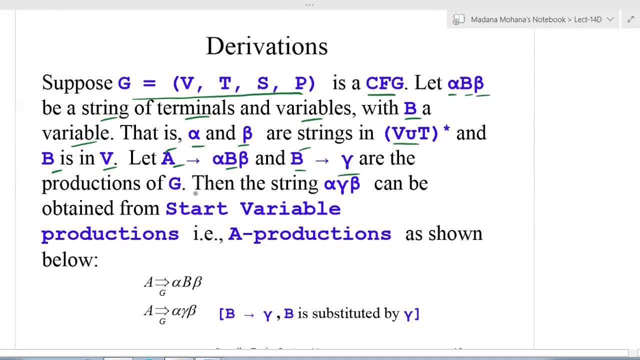 then b derives gamma. are the productions of g, then the string alpha, gamma, beta can be obtained from start, variable start variable production. that is a production as shown below now. here you can see the starting, the production: a derives alpha, b, beta. here we have substitution for b. 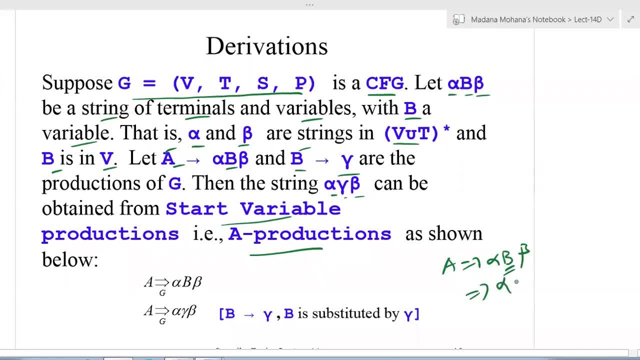 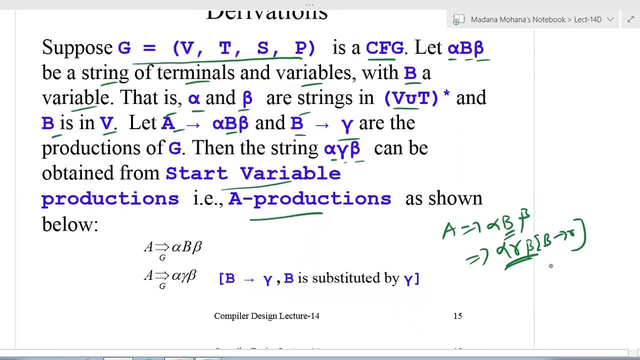 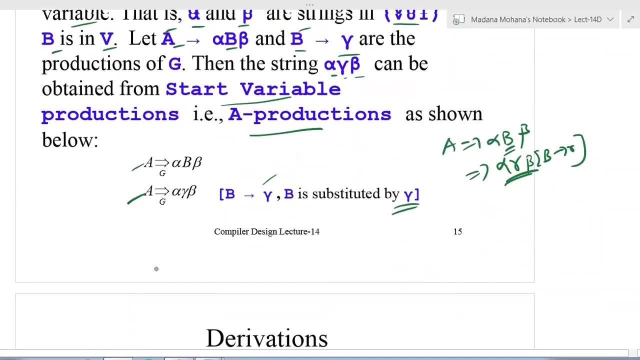 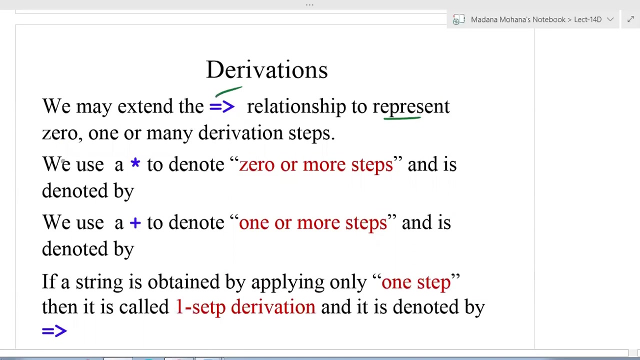 then you can substitute b productions. now this will become alpha b is substituted with gamma beta. here what we substituted b derives gamma is substituted. now we derive the string alpha, gamma beta. this is the concept of derivation. so here b, b derives gamma. b is substituted by gamma. this is called as a derivation. so now we may extend the derivation relationship to represent: 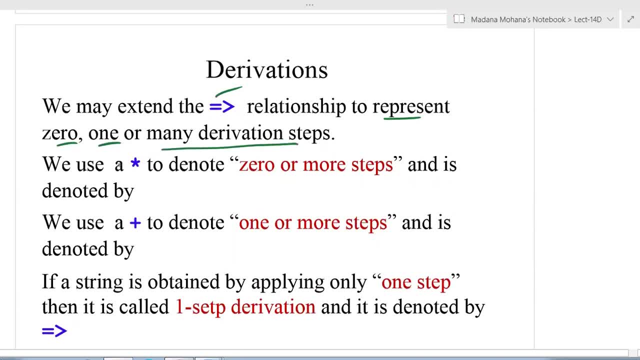 zero, one or many derivation steps. if we use asterisk to denote zero or more steps and is denoted by this one, then if we use plus to denote one or more steps, and if this is denoted by that symbol under place, Then this is denoted by the derivation symbol under a string. Now, 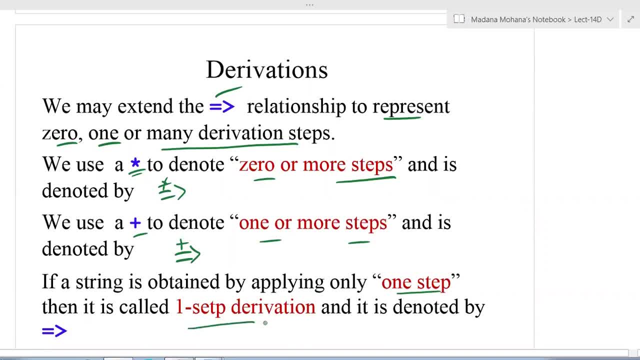 if a string is obtained by applying only one step, then it is called as one step derivation. This is simply denoted by the arrow, without positive closure or star closure. So these are all the various variants of derivations. So then, let us consider examples. So the same. 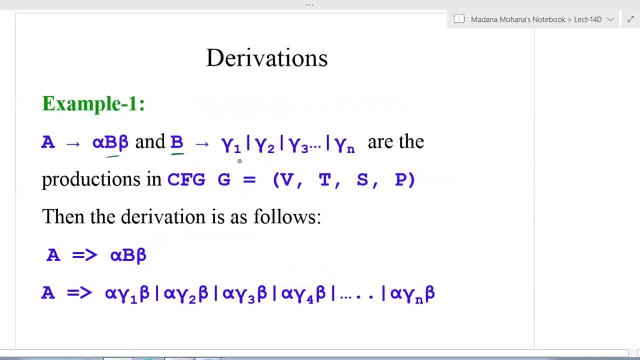 example what we discussed: A derives alpha, B, beta. Now B contains multiple production, That is gamma 1 or gamma 2 and so on. gamma n are the productions in the context to gamma G equal to VTSV. Then the derivation is as follows: First we can take the starting variable. 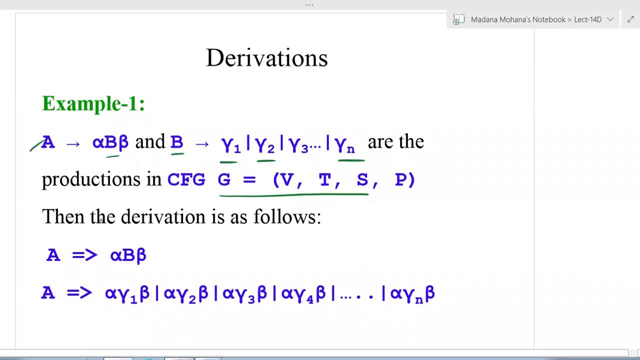 production A, The starting variable production A. So therefore A derives alpha, B beta. Now we have to substitute the B productions one at a time. Now A derives alpha, The first two B production is gamma 1. So here we have to substitute it: gamma 1 or alpha beta, no. 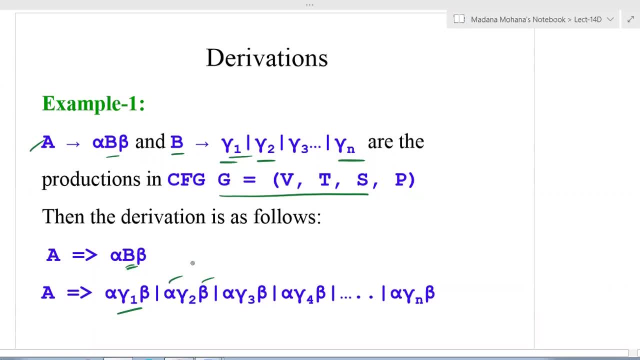 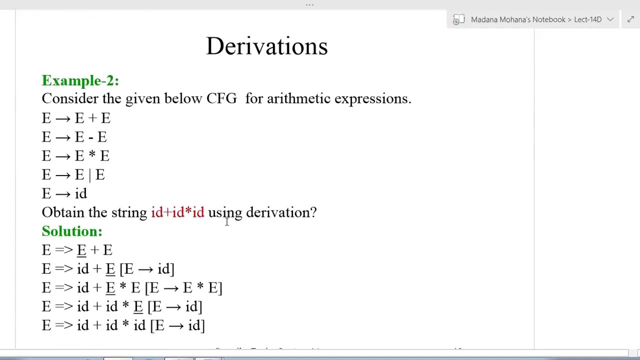 change Not changed. Only gamma B value is changed with gamma 1 to gamma n. Now second production here gamma 2,. third one, gamma 3, and so on gamma n. So now this is called as a derivation, Like that we have to derive a particular string or some partial derivations. 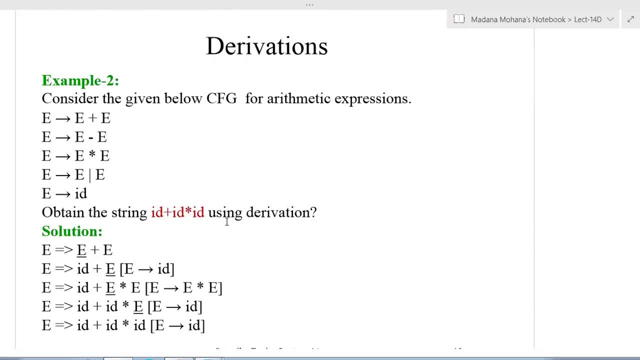 by substituting The corresponding productions. So another example: Consider the given CFG for arithmetic expression. Here this is the arithmetic grammar. This we already explained. Now we have to derive the string ID plus ID into ID using the derivation. So here all the productions. 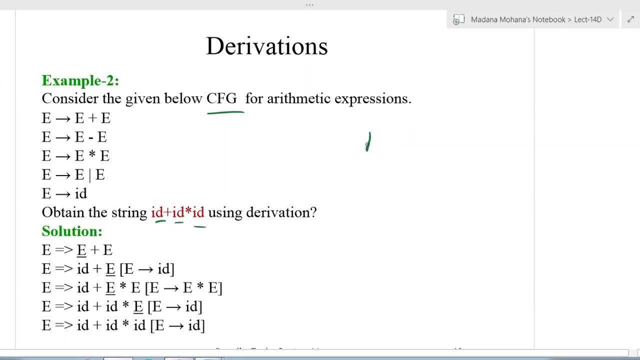 starting with same variable only. You can take any variable. Suppose let us take E derives E plus E. So here your string contains plus and into. So first left part We have to consider Plus, Then right part you have to consider into. Now this will becomes: 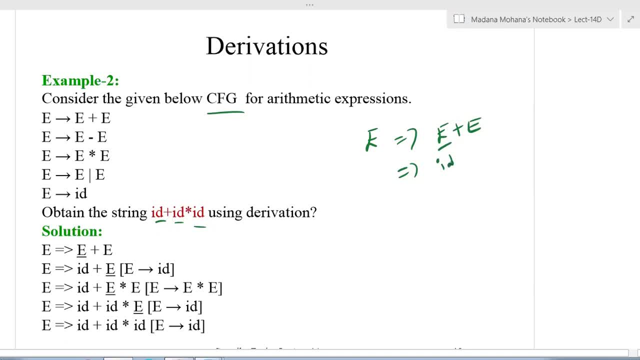 here leftmost E, you can substitute with ID, then plus E. Here what we substituted, E derives ID, Then after ID: plus what do you want? Again? ID into Now. in place of E you can substitute INTO production For INTO production. we have E derives E into E. Now this will become: 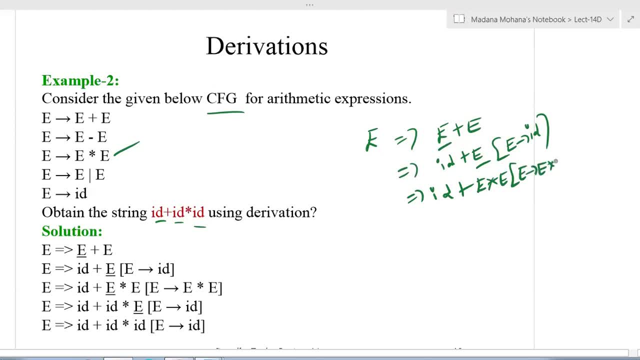 E into E. Lo****–田 E into E Here. what we substituted In here for E and E derives into E. This will become at: e derives e into e now. then, in place of e again, you can substitute id. now this will become: 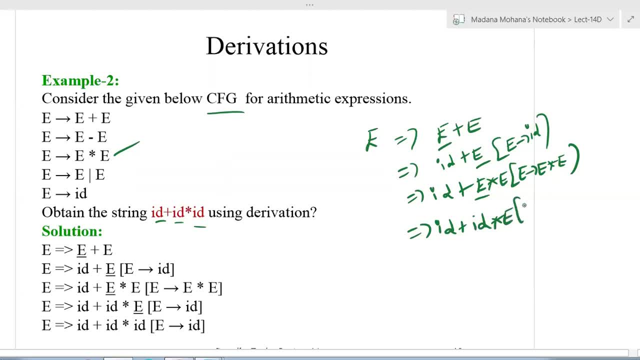 id plus id into e. here, what we substituted e derives id. now, at last, one more e is there again. you can substitute that e by id. now this will become id plus id into id. now here, what we substituted e derives id. so this is your required string. so like that, we have to derive the string. 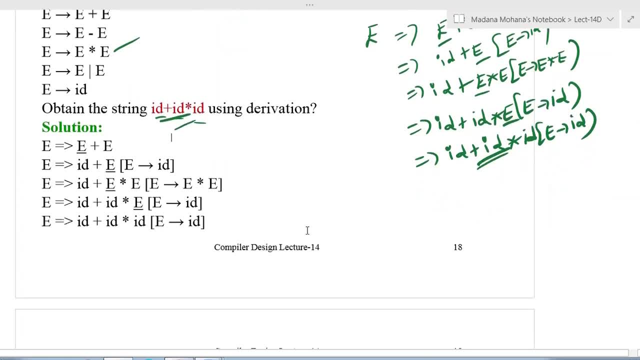 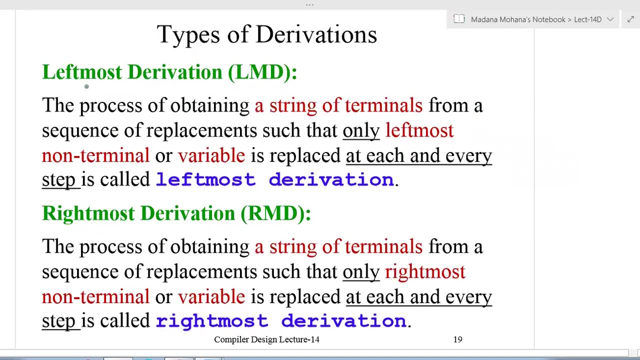 by applying respective productions. so now types of derivations. so there are two types of derivations. the first one is called as leftmost derivation, then the second one is called as rightmost derivation: the process of obtaining a string of terminals from a sequence of replacements such that only leftmost non-terminal or variable is replaced at each and every step. this is called 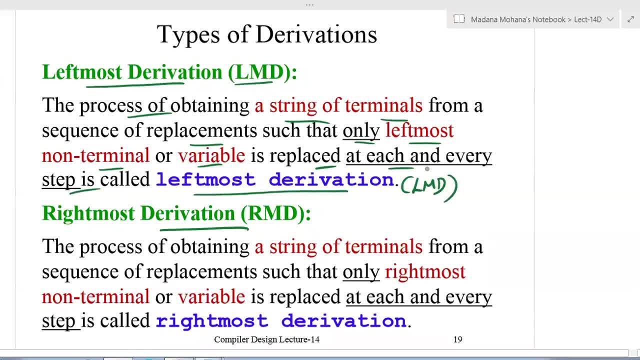 as leftmost derivation. so in the process of obtaining a string of terminals from a sequence of replacements, the process of derivation in the right hand side, leftmost variable, we have to replace first each and every time that is called as leftmost derivation, whereas rightmost derivation simply the reverse, the process of obtaining a string of terminals from a 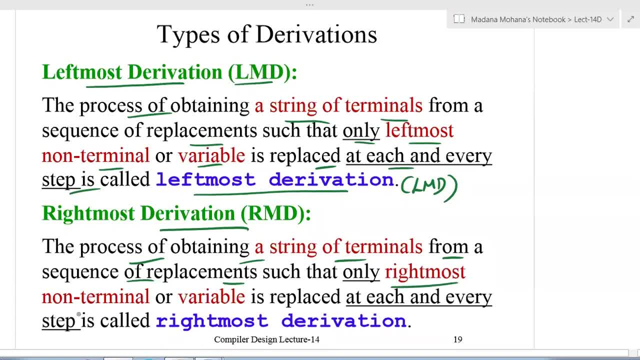 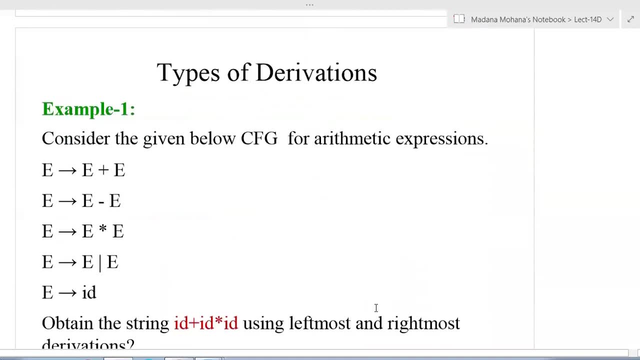 sequence of replacements such that only rightmost non-terminal or variable is replaced at each and every step, is called as rightmost derivation. now the previous example we have to recall. now we can apply both the leftmost and rightmost derivation. the same example you have to consider. consider the. 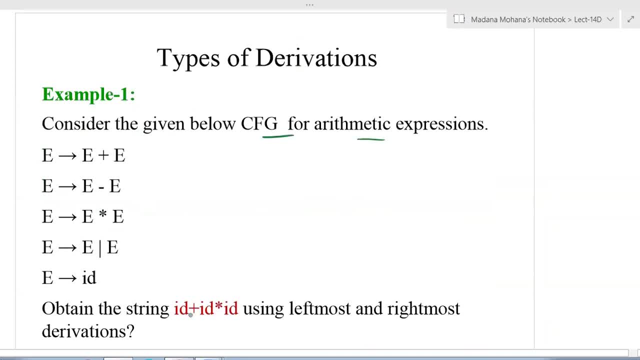 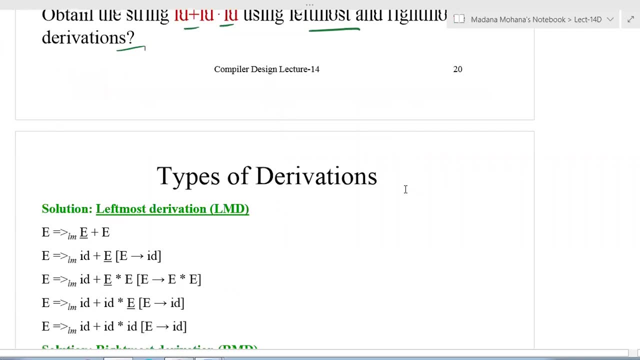 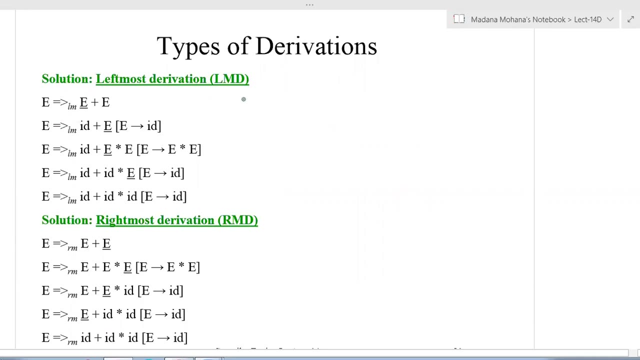 given cfg for automatic expression. now obtain the string id plus id into id using the leftmost and rightmost derivations. now let us see the two derivations here. you can start with any production because all are starting with the same starting variable, e, suppose here. now let us see. 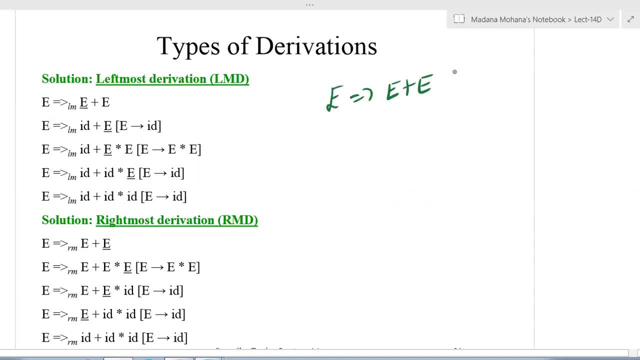 e derives, e plus e is taken. so whenever you can apply leftmost derivation, here you can prefix with: lm stands for leftmost derivation. so every time here see two variables, are there variable one, variable two, the leftmost variable. first, this you can replace. so now here this is: 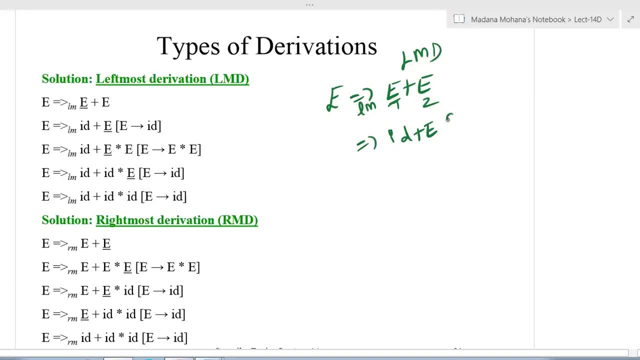 replaced with id plus e. now here what we did: e derives id is substituted. now here only one variable is substituted. so here only one variable is substituted. so now here only one variable is there. directly you can substitute more than one variable means then you can substitute leftmost. 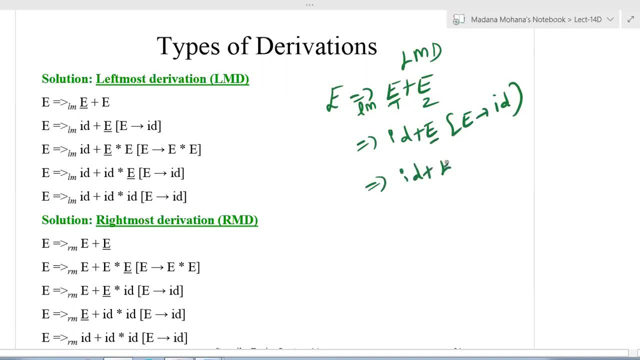 variable first, now id plus. now this e is substituted with e into e. now, here, what we substituted e derives e into e. now here two variables are there. so leftmost variable: we have to substitute: now id plus, now id into e. here what we substituted e is substituted with id now. 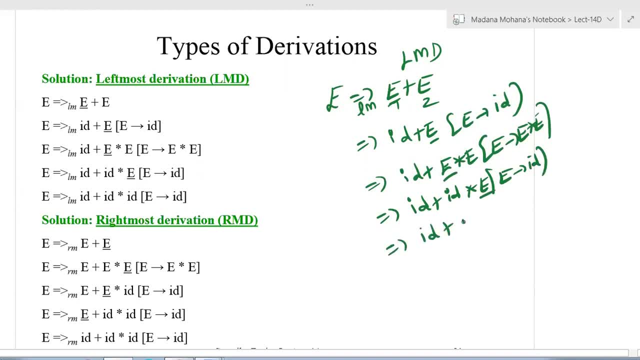 only one variable, e is there. you can substitute with id only. so now this is the leftmost derivation. the previous example: whatever we explain by default, that is leftmost derivation. now say we can apply for rightmost derivation. now here you can see: e derives e plus e. now rightmost e this: 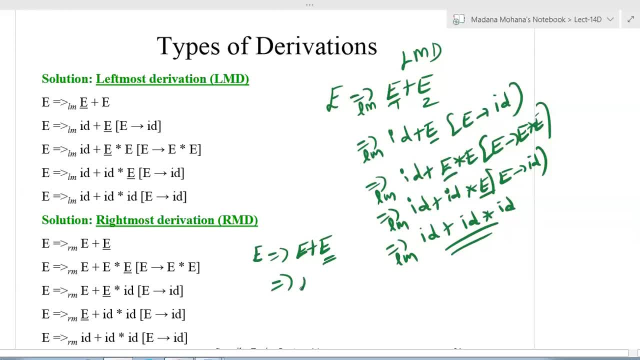 you can substitute first now here after place, what you are, what you have, you are having in the state, so you have to. so you can substitute this by e. now here, what we substituted e derives e into e. now here three variables are there. rightmost variable you can substitute first now. this will become e plus e. 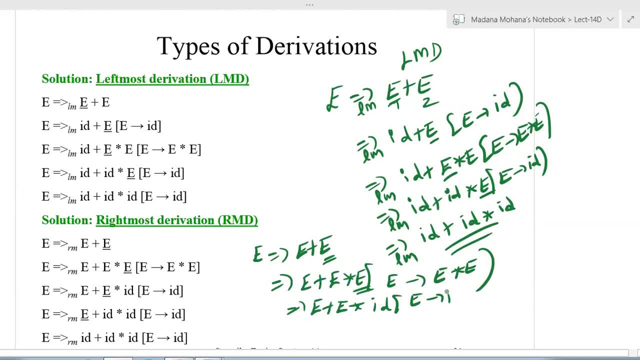 into now id. now e derives id. now again, two variables are there. rightmost e you can substitute first with same id, e plus id into id. now here we substituted id in place of e. now then at last one more: e is there. now you can substitute id, id plus id into id. here what we 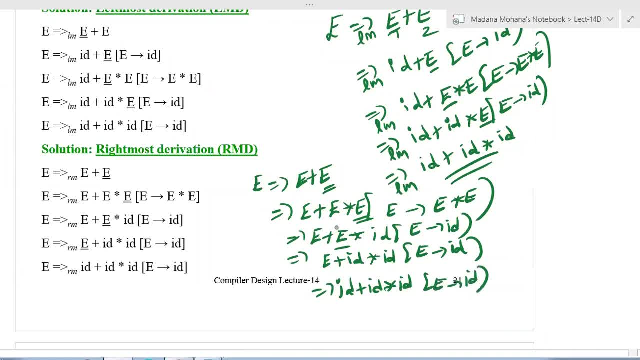 substituted e derives id. now you can see, here this derivation is different from the previous derivation which is called as rightmost derivation. here you can make the label as rm, so now. but here we derive the same string here also. so these are all the leftmost and rightmost derivations. then coming to 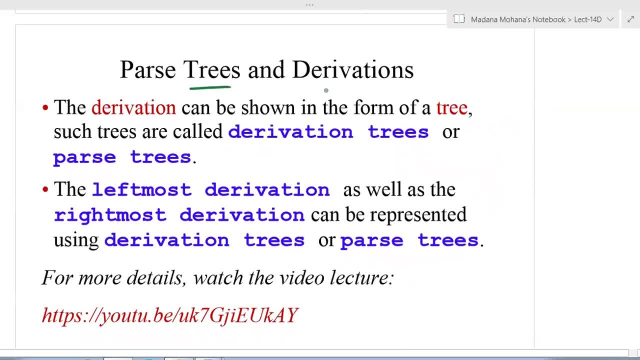 the derivation tree, then derivations, parse trees and derivations. the derivation can be shown in the form of a tree. such trees are called as derivation trees or parse trees. the leftmost derivation as well as the rightmost derivation can be represented using derivation trees or parse trees. the concept: 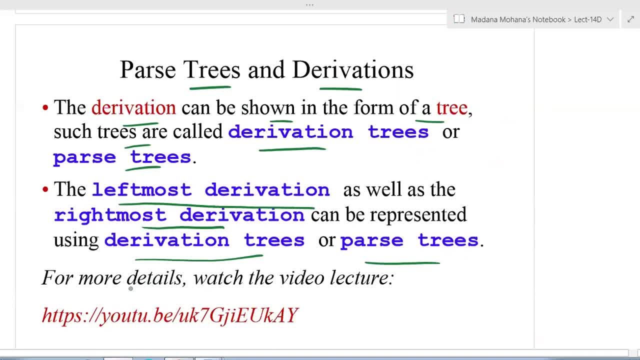 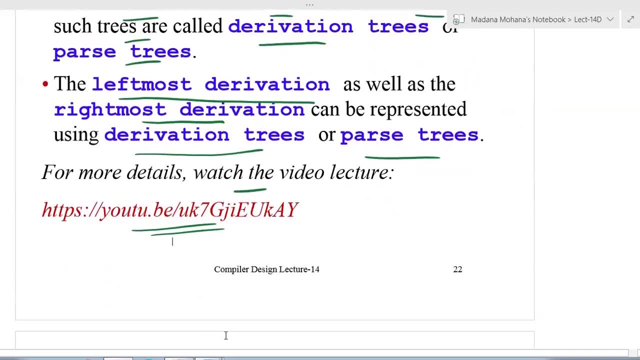 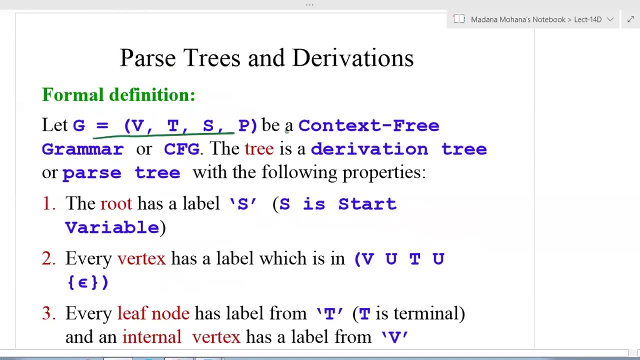 of this, derivation trees are parse trees. for full lecture, you can watch the following video where we discuss it in the course formal language and automata theory. so now formal e: how to define the parse tree or derivation tree. let g equal to vtsp be a context grammar. 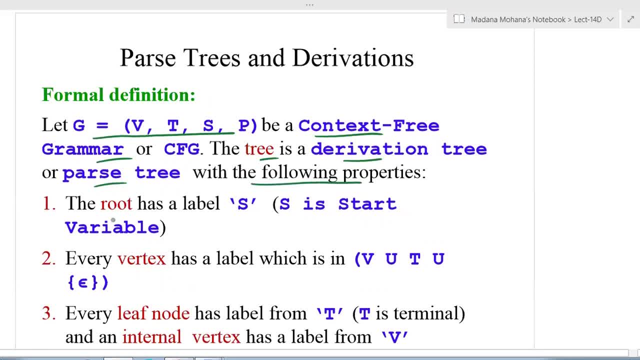 the tree is a derivation tree or parse tree with the following properties: the root has labeled with starting variable capital s. then every vertex has a label which is in v, union, t union, null. so every vertex is labeled with the combination of either variables or terminals are possibly null. then every leaf node has a label from terminal. 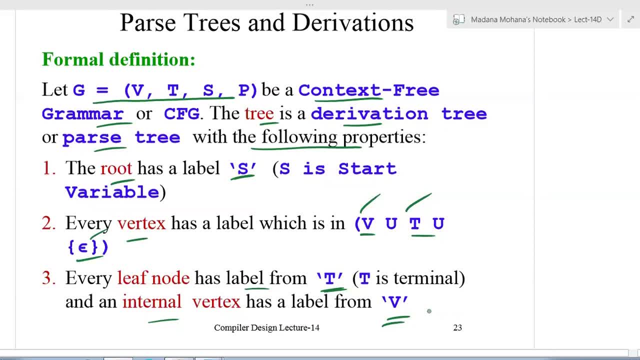 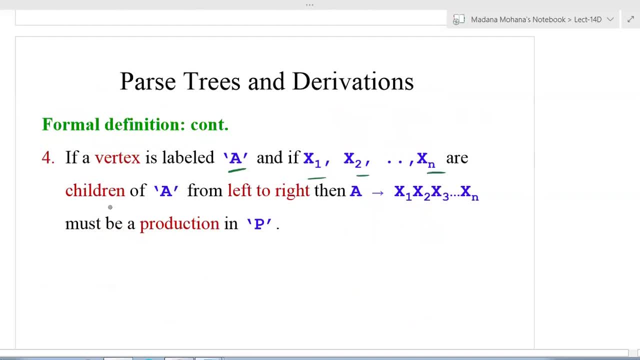 and internal vertex has a label from variable. then if a vertex is labeled with a and if x1, x2 and so on, xn are children of a from left to right, then a derives x1 to xn must be the production in p. suppose here a vertex is labeled with a, then we have the children's x1, x2 and so on, xn, these 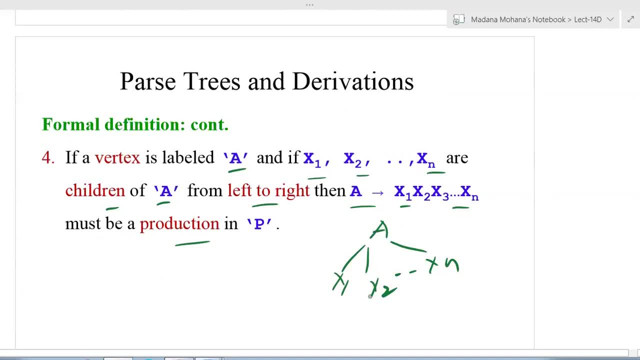 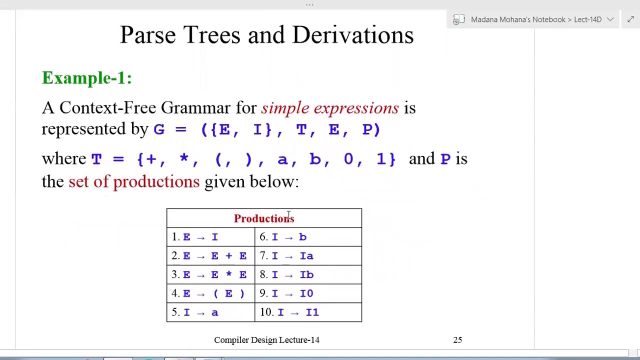 are all connected to that node, a from left to right as children's. when this is possible, whenever this production, a derives, x1, h turns on, xn must be production in p. so generally this is possible. now let us consider the previous example. so a context with grammar per simple expression represented by g equal to 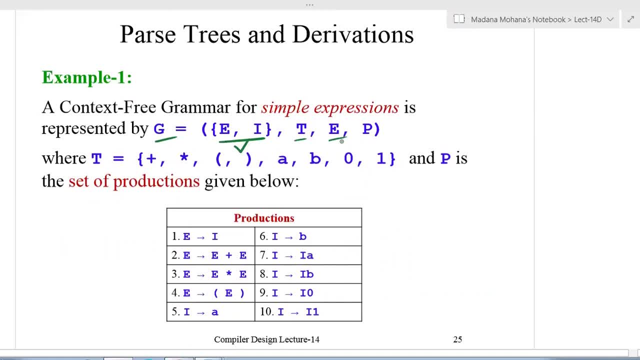 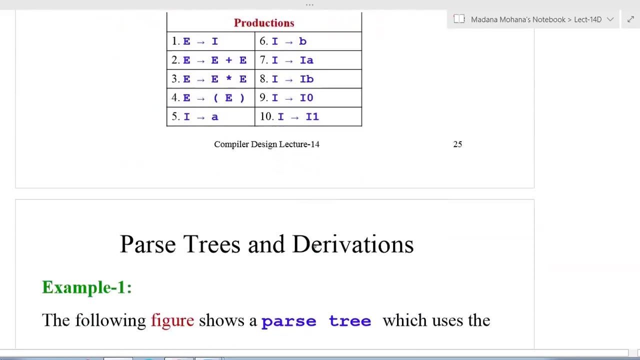 e, comma, i. these are all the variables now. t terminals, then e is the starting variable, p productions, where t equal to plus into left parentheses, right parentheses, is small, a small v, 0, 1, or the terminals and productions are given below. now these are all the productions. now we have to construct a derivation tree or parse tree, the following: 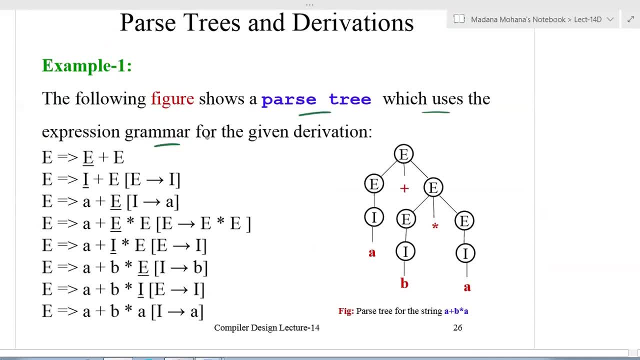 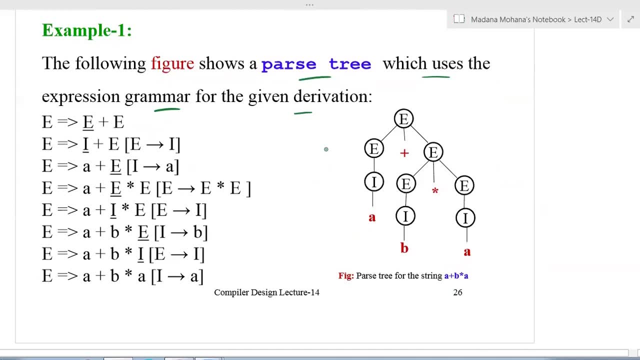 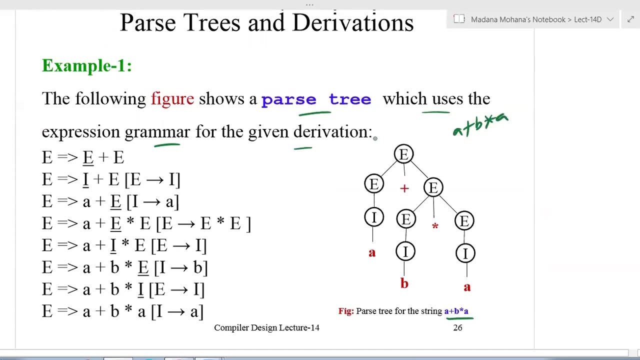 figure shows a parse tree or derivation tree which uses the expression grammar for the given derivation. so now here we derived the string a plus b into a, a plus b into a. first you can find out derivation for this string. then, automatically, using the derivation, you can construct its equivalent derivation tree or power stream. now you want. 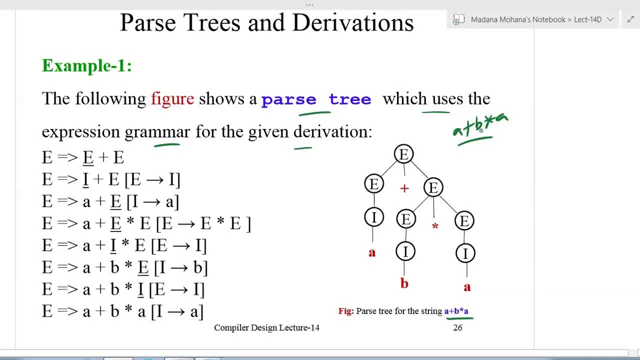 to derive a plus b into a, like id plus id into a in a similar fashion. first leftmost part- we are having place. we can take the production related to place. so we have taken here what we have taken. he derives e plus e. production is taken now if 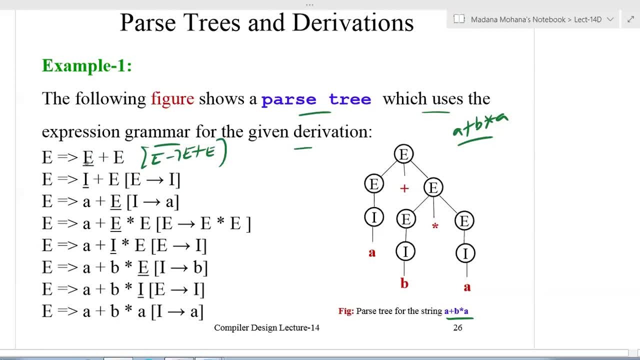 we can apply leftmost derivation or any derivation you can apply, so here, leftmost variable. so what e contains e contains e i. so this is the production in the given grammar: e derives i. now i contains terminal a. you can substitute a. now we got a place then what you want to be into, a. 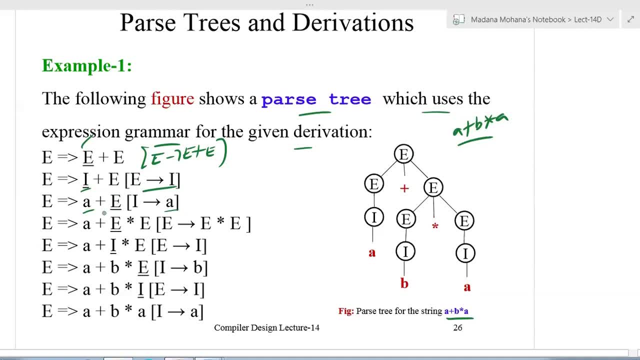 so then latter part: you want multiplication. so in place of e you can substitute the multiplication production. now e is substituted with e into e. this is the production we are having. e is replaced with i, then i is replaced with b, then now we got b, so a plus b into then at last. 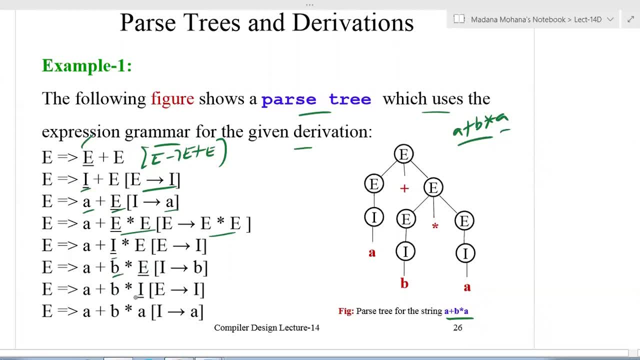 what you want. terminal a, now e is again substituted with i, then i is substituted with a, now a plus b into a. this is our required string now. stepwise, whatever the substitution we used in the derivation, same we will consider the leftmost starting variable. you can consider it as the root now. this is the root. 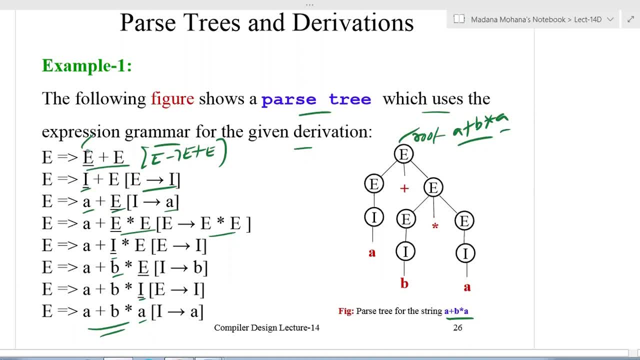 now first what we did. e is substituted with e plus e, so it is in the form of x1, x2 and so on. xn, a directs x1 to xn. all are children's of a connected to a from left to right. now e plus e. you can connect to from left to right to the root e. now e plus e. now then what we did next: leftmost. 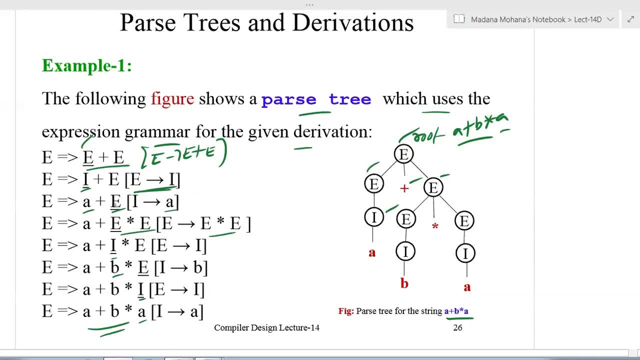 e is substituted with i, then what we did leftmost i is substituted with a, then what we did next: e, that is replaced with e, into e. so here this e is replaced with e into e, then this leftmost e substituted with i, then the substitute with b, then this is substituted with i, then substitute with a. 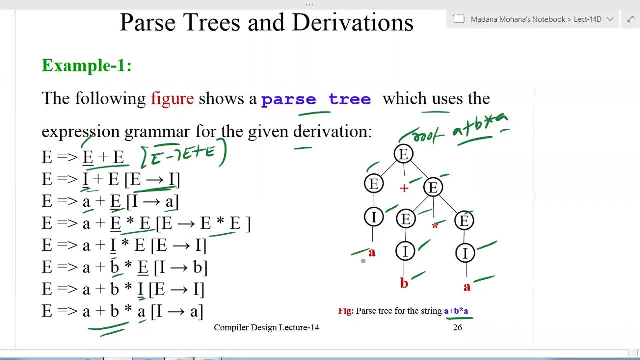 now you can take all leaf nodes from left to right. here you can see a plus b into a. now here, a plus b into a, one, two, three, four, five. so if any null, is there any leaf node, conditional, you can exclude null. now this is our required string, which is called as: 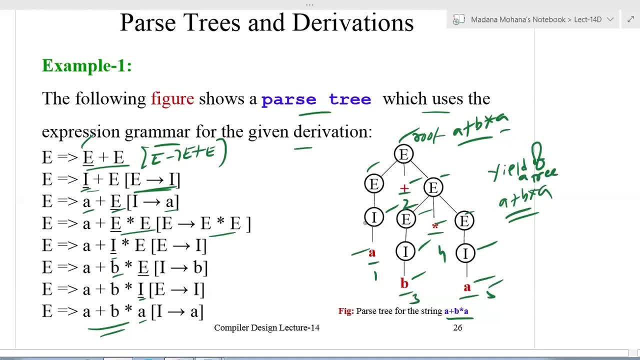 yield of a tree, yield of a tree so from the derivation tree or parse tree, by considering all the leaf nodes from left to right, excluding null, then whatever the sentence or string will obtain that is called as yield of a derivation tree or force tree. now, this is the way of construction of derivation. 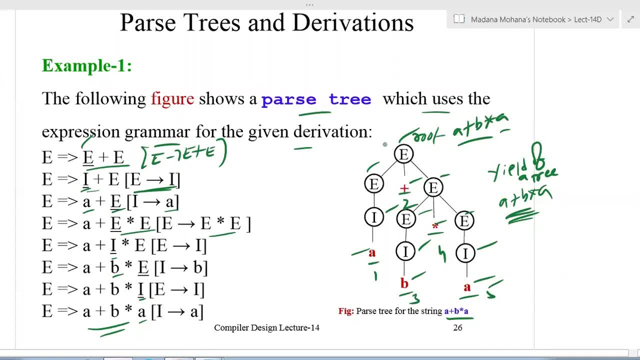 so from the derivation of meinen rules you can observe that these leaf nodes are divided into Ä and Ö. this is our Gangly grupo matrix of the thing, both EÄ and Ö, differentıy that you can observe. all the variables are represented within the circle 완I� ab savory necesidadpot Paw streak. here you can observe all the variables. that was. 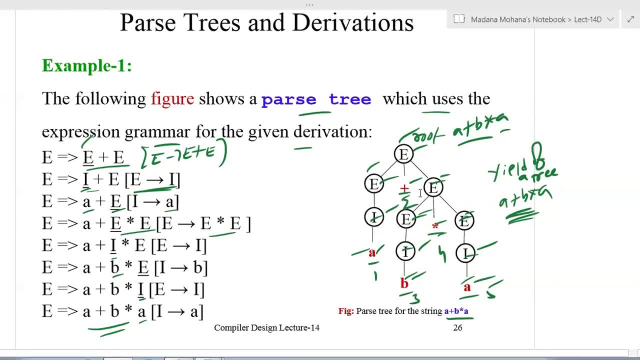 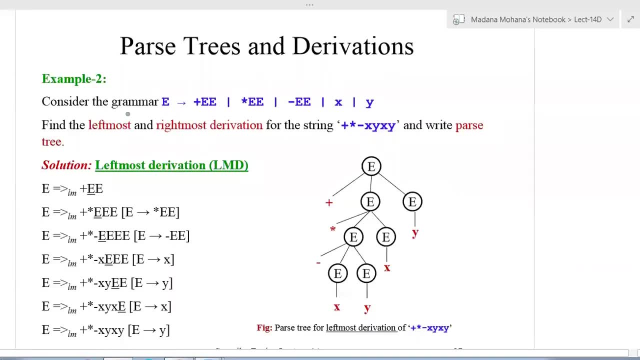 terminals. no expansions are possible further. So these are all the notations used in derivation tree or parse tree. So similarly, another example: consider the grammar: ee derives plus ee or into ee, or minus ee, or x or y. Find the leftmost and rightmost. 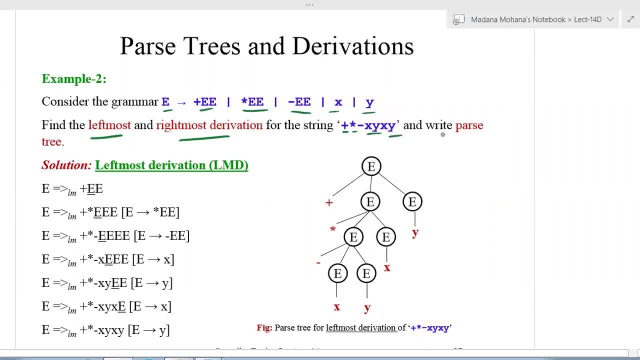 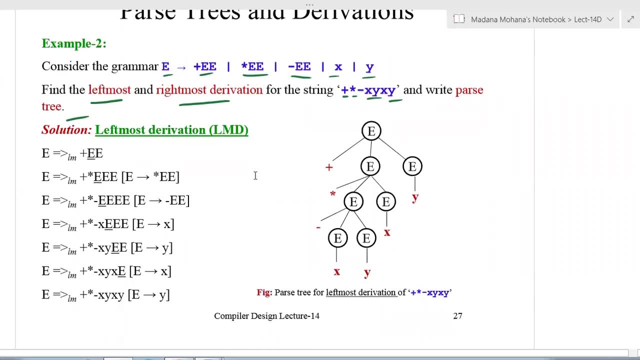 derivations for the string plus into minus, xy, xy, and write parse tree. So you can do in the similar manner. So here they mentioned, to find the leftmost derivation and rightmost derivation. So for every derivation you can draw the corresponding derivation tree. or 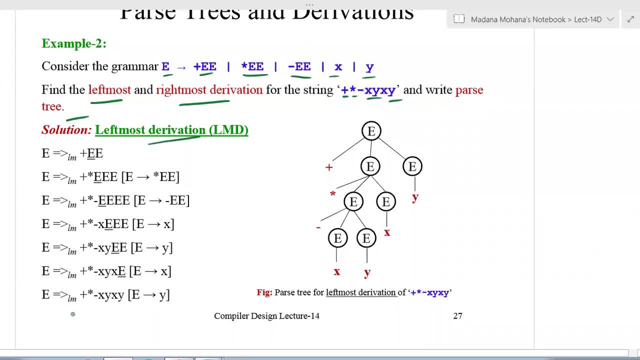 parse tree. Here this is the leftmost derivation in the same process. So finally, whatever the substitutions we used, those are all represented in bracket, So those you can substitute in the derivation tree also to derive the string. Now here you can take all the leaf nodes. 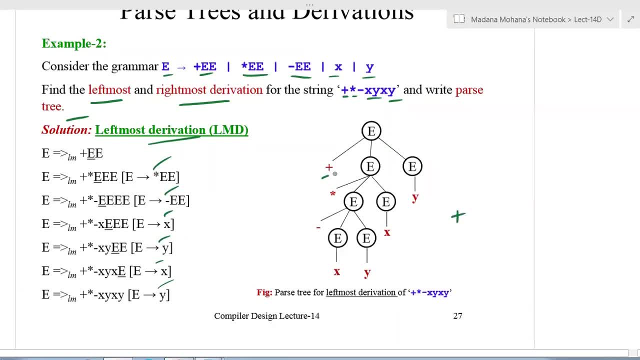 from left to right. So here you can see: first is the string, So first is plus, then into next one is minus. next leaf node is x, next leaf node is y, next leaf node is x, next leaf node is y. Now you can see. this is your required string plus. 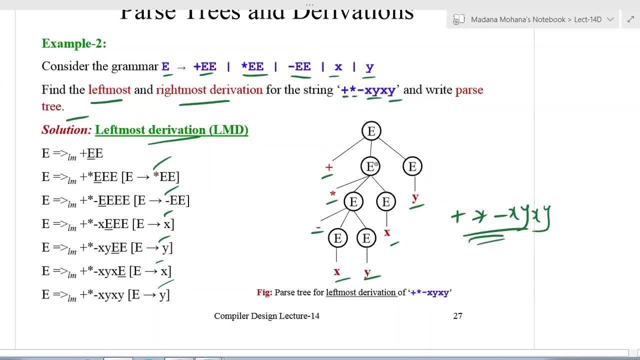 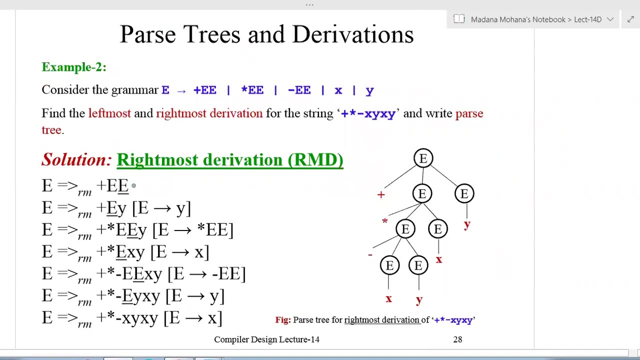 into minus xy, xy by connecting all leaf nodes from left to right. This is called as yield of a derivation tree or parse tree. This is the derivation tree corresponding to the leftmost derivation. Similarly, rightmost derivation, so rightmost derivation, every time rightmost. 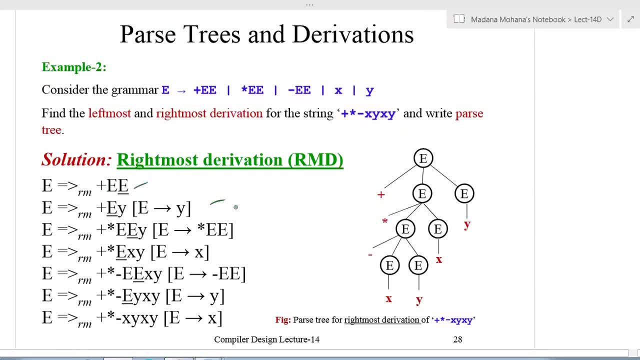 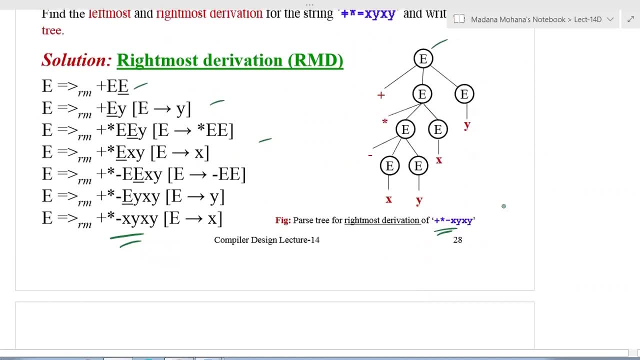 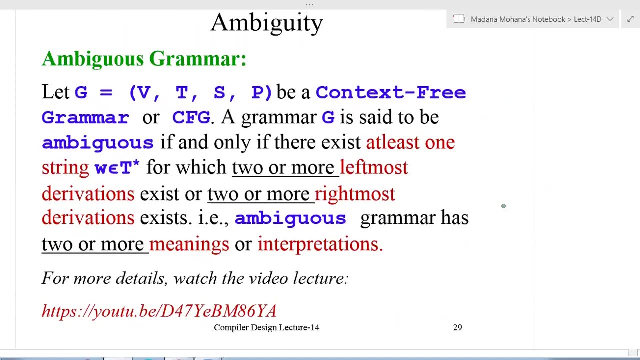 variable is substituted first. So this is the rightmost derivation. Now here we got the same string. now this is the derivation tree, or parse tree for rightmost derivation. Now, next concept is ambiguity. So when you can say a grammar is ambiguous, Let g equal. 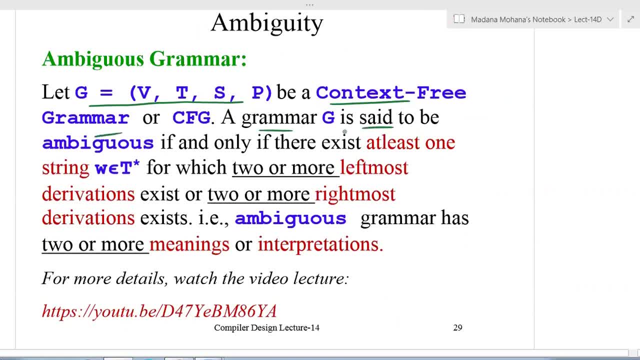 to vtsp be a context-free grammar. a grammar g said to be ambiguous. the condition is if, and only if, there exists at least one string. w belongs to tau closure, which is a string of terminals for which two or more leftmost derivations exist, or two or more rightmost derivations exist. that is ambiguous grammar has two or more. 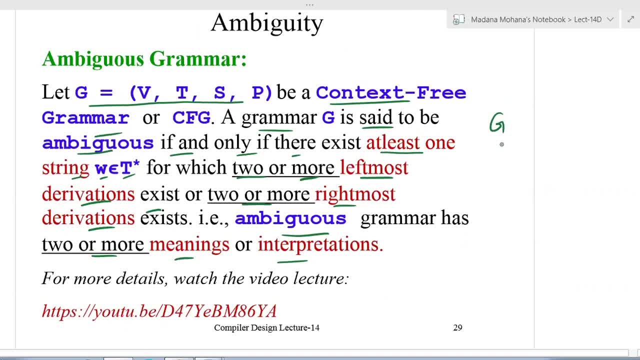 meanings or interpretation. so for a contextual grammar g, two or more leftmost derivations for the string w or two or more rightmost derivations for the string w. now the grammar is said to be ambiguous, the grammar having ambiguity, the concept of ambiguity. so where we studied, 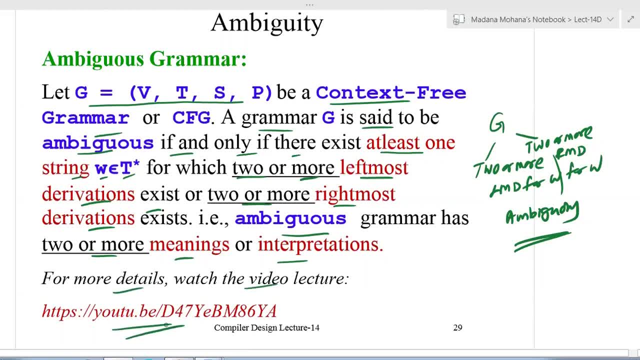 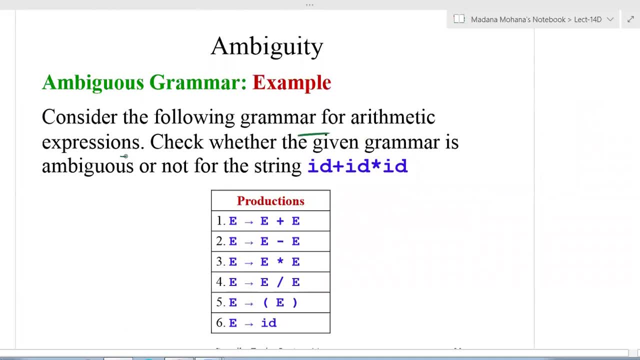 in the course formal language and automata theory. you can watch the following lecture for more details. So now let us consider an example. Consider the following grammar for automatic expression: check whether the given grammar is ambiguous or not for the string id plus id into id. So in exam basis sometimes you will get this type of questions. check. 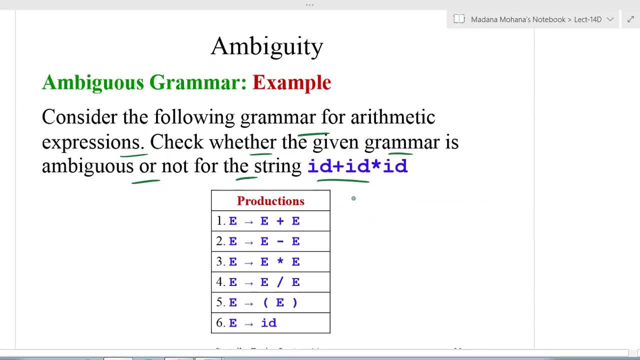 whether the given grammar is ambiguous or not, for one string. So what you have to do for that string you need to find out minimum two leftmost derivations which derives the same string, or two rightmost derivations, any one type of derivation. if you can find that's. 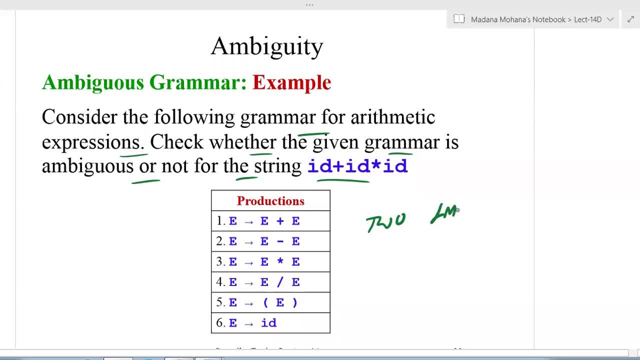 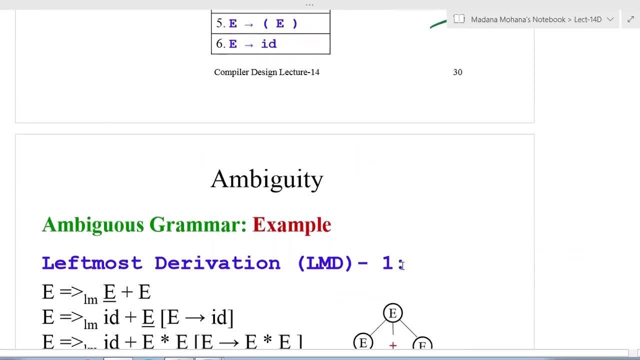 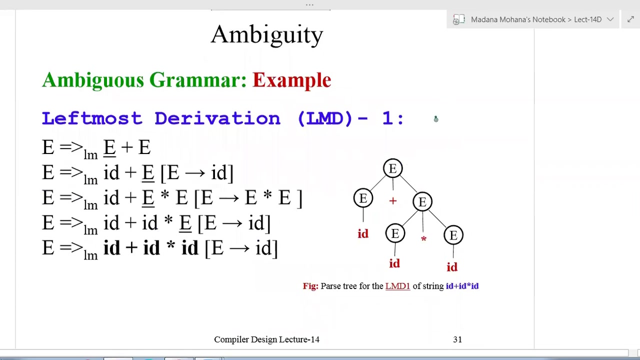 enough, either two leftmost derivations or two rightmost derivation, any one you can use, but then which derives the same string in both cases? then you can say: the grammar is ambiguous grammar. Now let us see here: First for the string id plus id into id, here for the string id plus id into id. this is leftmost. 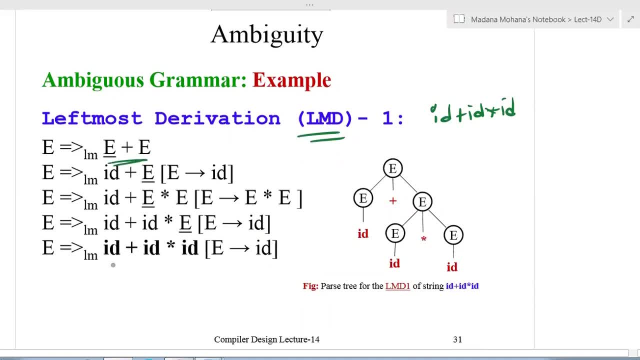 derivation one. here we have taken e derives e plus e. now finally, here we derived id plus id into id. now the corresponding derivation is also constructed. here you can take all leaf nodes from left to right, id plus id into id. now we got the string. So this is lmd one. 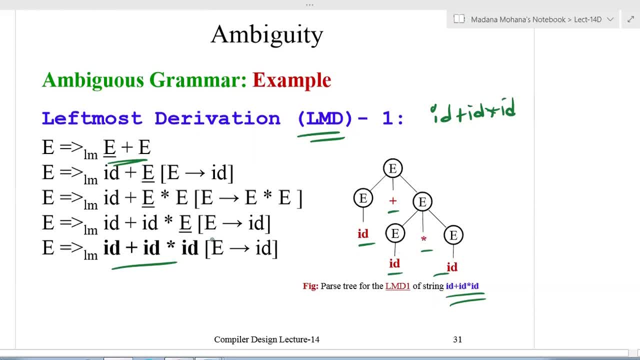 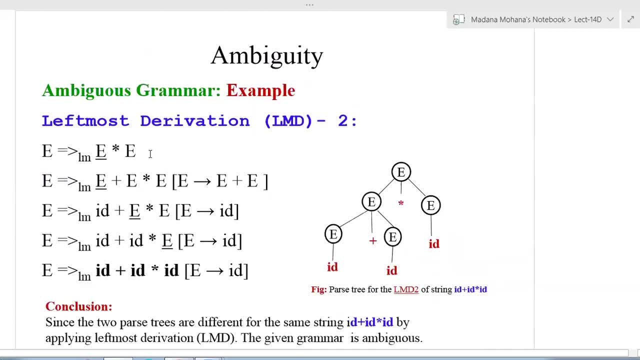 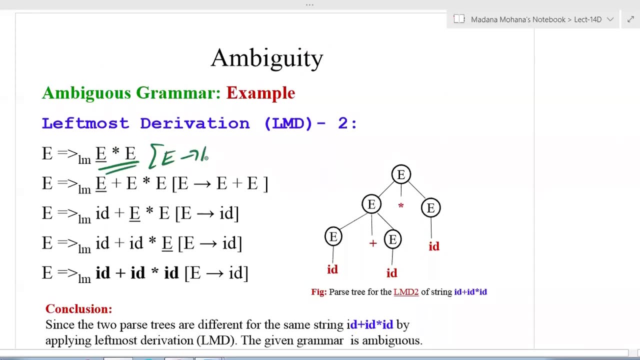 first your derivation tree. Now let us take another starting production. here we started with e plus e. now if we can take other than e plus e, now you can see, here we have taken e into e. this is a different production than e plus e. So here we substitute e derives e into e In the first step itself. 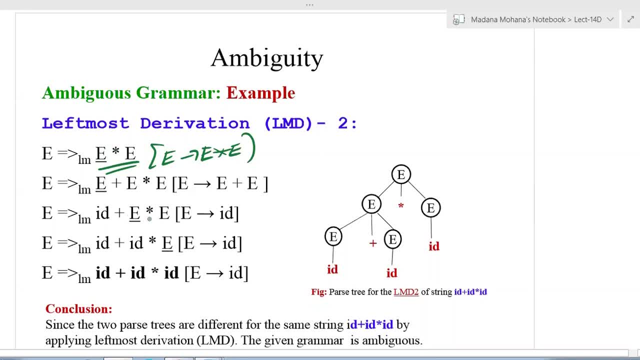 so the derivation is changing now by applying leftmost derivation every time leftmost variable is substituted first. Then here We derived id plus id into id, id into id. now for this the derivation tree. here you can see, you can take all the leaf nodes from. 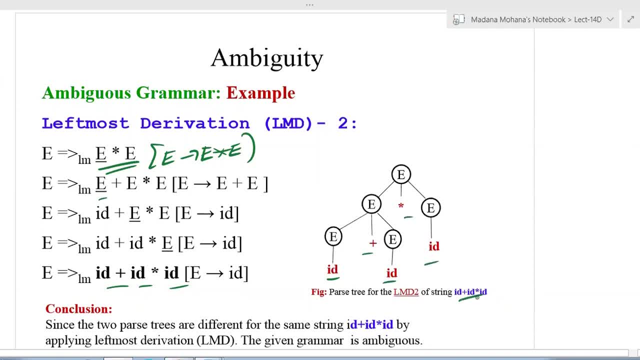 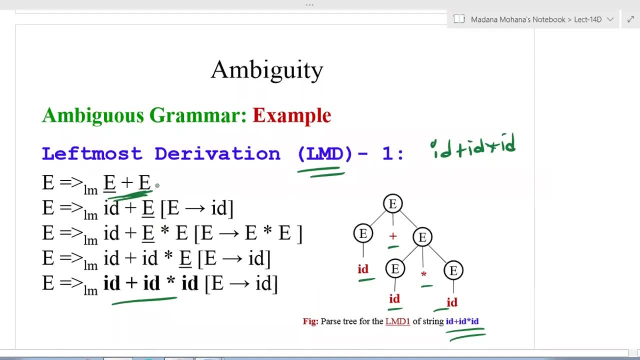 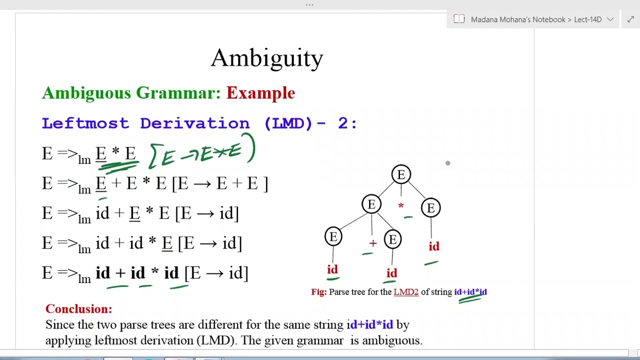 left to right, id plus id into id. so we got the required string. now you can compare lmd1 and lmd2. so lmd1 starting with e plus e, now the derivation tree, also the second level. here it has e plus e. then here this is e. now here you can see. here it is changing. here e into e, is there. 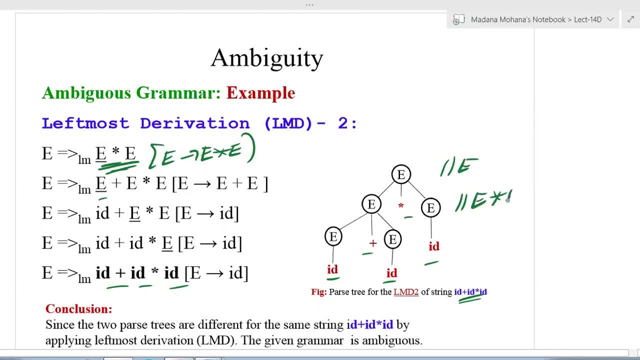 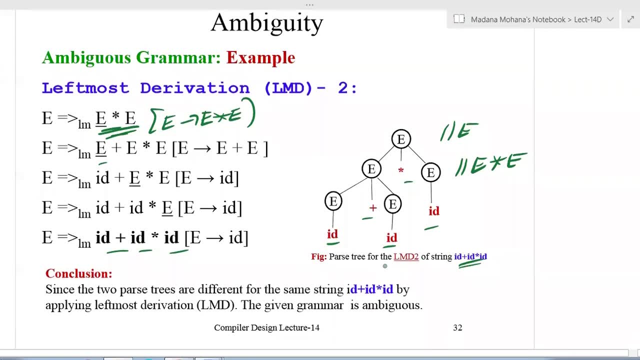 so here e, so here e into e. so now both the derivation and derivation trees are different, but there is the same string. therefore, as for our definition of ambiguity, so the grammar is ambiguous. so, since the two parse trees are different for the same string, id plus id, into id. 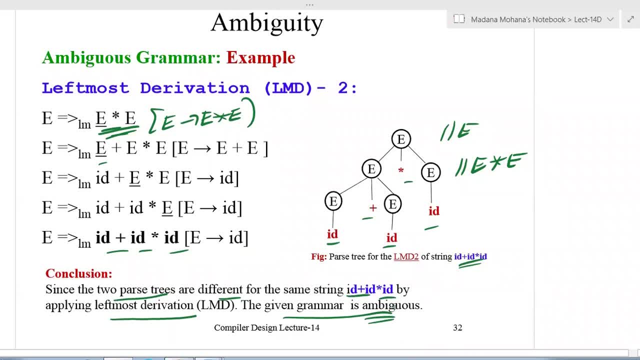 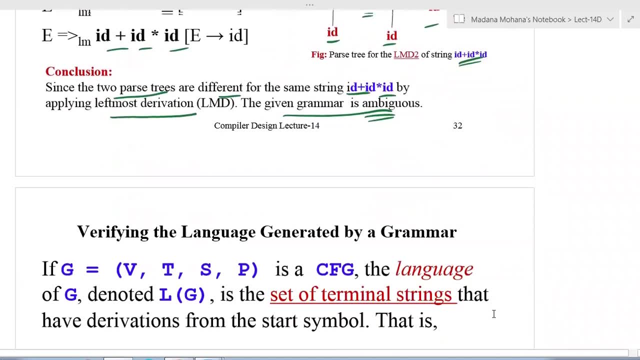 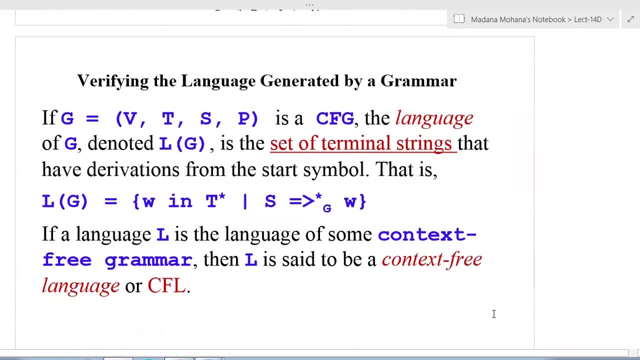 by applying left one derivation, so the given grammar is ambiguous, then you can apply rightmost derivation also, that you can do it as a practice problem, so like that we can check whether the given grammar is ambiguous or not. then, moving to next concept: verifying the language generated by a grammar. 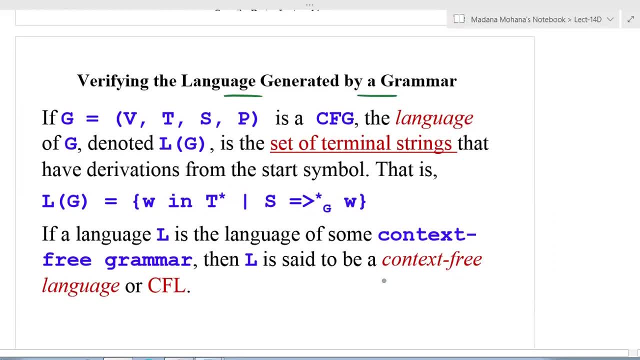 so nothing but from the grammar. so whatever the strings you are deriving based on that, you can generate the language generated by the grammar, which is denoted by l of g. so g equal to vtsp is a context grammar. the language g denoted l of g is the set of terminal strings that have derivations from: 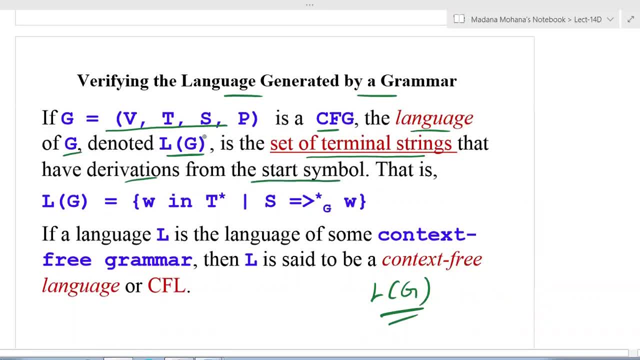 the start symbol. so here the language consisting of only string of terminals only. so therefore this is defined as l of g equal to w in t, closer, that is, string of terminals. so now these string can be derived from the starting order of the string. you can see from the starting order. 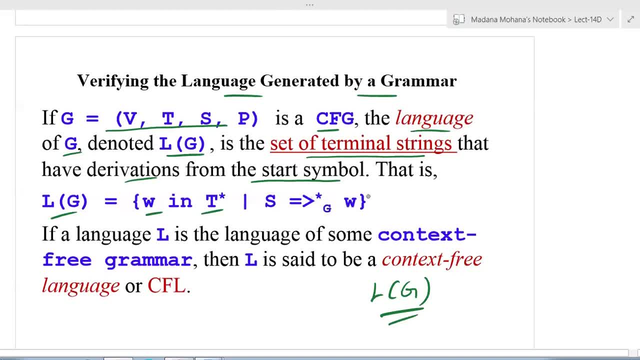 variable of the production, that is, S, derives W. So under ASTIC 0,, 1 or more substitutions are used then for from the grammar G. If a language L, if a language L is the language of some context free grammar, then L is said to be context free language, or CFL. So this: 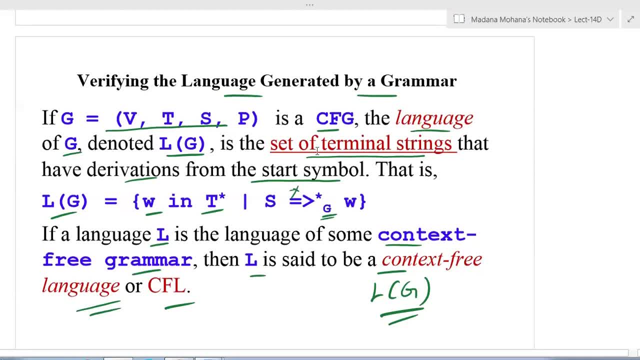 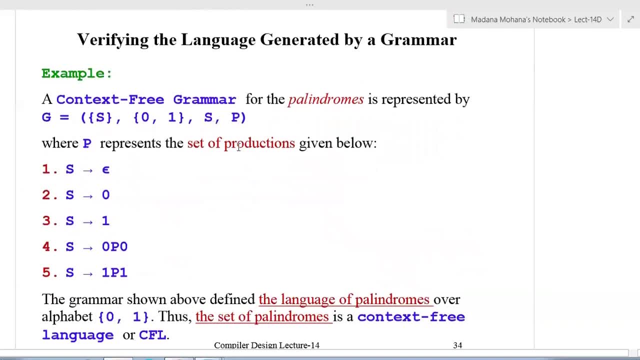 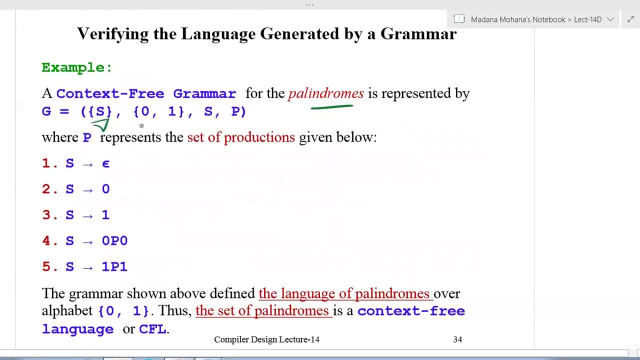 is the way of generating language by a grammar. So then, with this we can verify whether the language is generated by the grammar or not. Then let us see one example. A context free grammar for palindrome strings is represented by G. equal to S means V. Now 0 comma 1 are 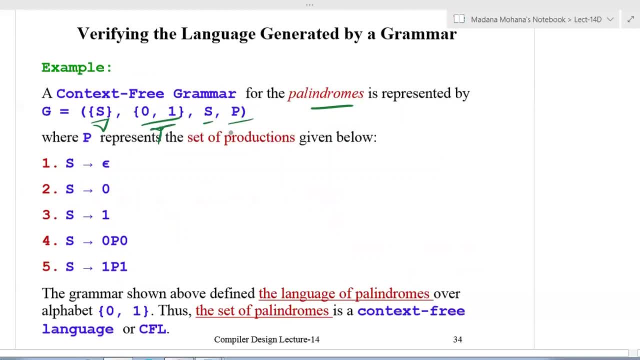 terminals T. Now S is the starting variable, P is the set of productions. The productions are given below 1 to 5 productions. So now, this grammar shown above defined the language of palindromes over the alphabet 0 comma 1.. Thus the set of. 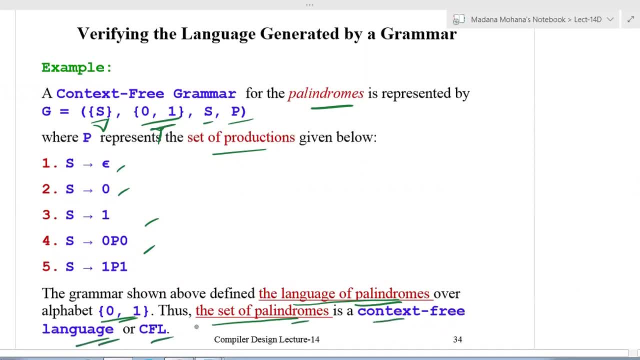 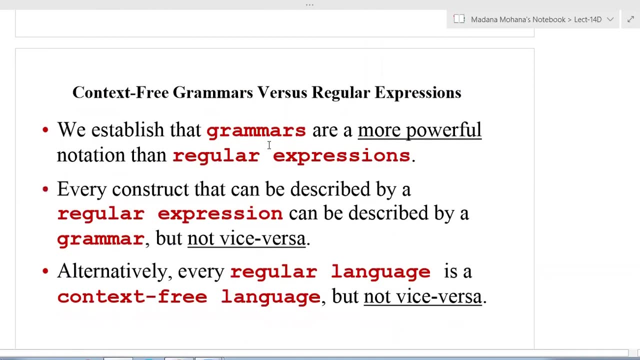 palindromes is a context free language or CFL. Therefore, L of G is context free language. Like that, you can verify language generated by a grammar. Now let us move to the last concept: context free grammar versus regular expression, CFG versus regular expression. 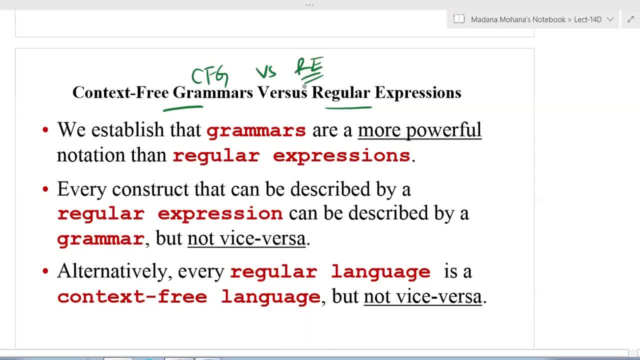 So now CFG 0, comma 1, we studied regular expression. we studied in our previous chapter under lexical analysis or scanner. now here we established that grammars are more powerful notation than regular expressions. every construct that can be described by a regular expression can be described by a grammar. but 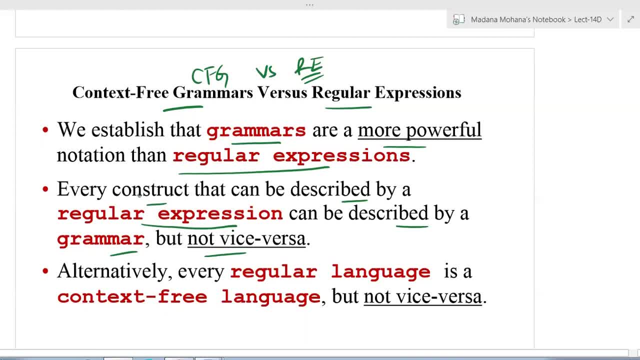 not vice versa. reverse is not possible, for every programming language construct that can be described by regular expression can also be described by grammar, but not vice versa. reverse is not possible. alternatively, every regular language is a contextual language, but not vice versa. that means every contextual language is not a regular language. reverse is not possible. 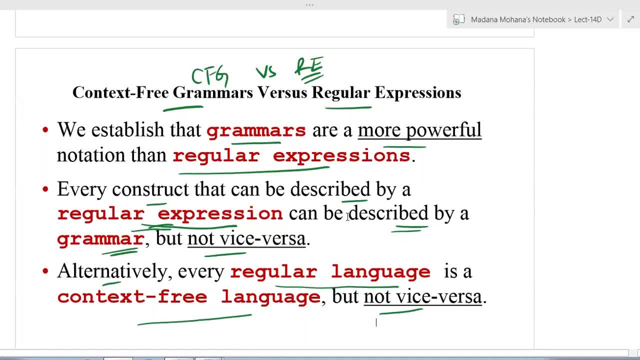 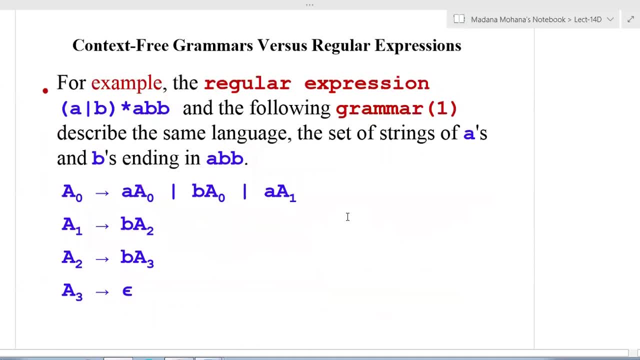 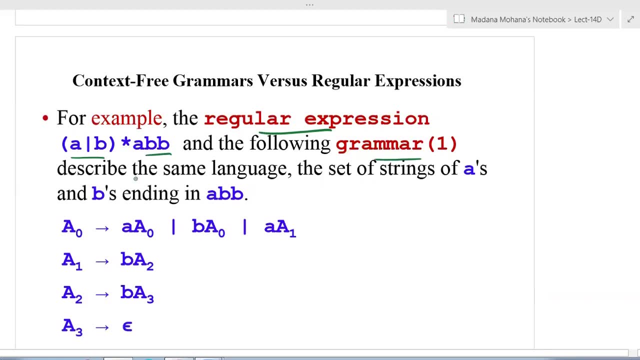 these are all some of the relationships among contextual grammars and regular expressions. now let us consider one example. for example, the regular expression a plus b, whole closer, a, b, b and the following grammar describe the same language, the set of strings of a's and b's ending with a, b, b. so this regular expression describes the language. 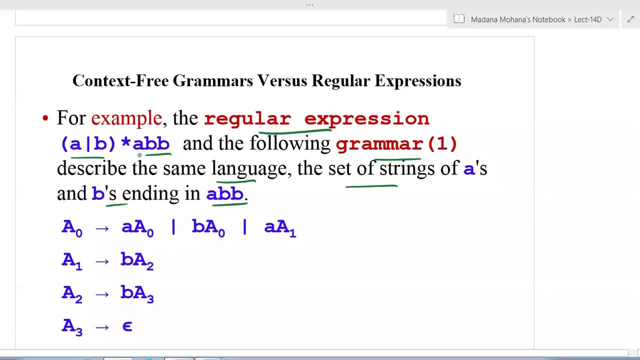 of strings of a's and b's ending with a, b, b. so now this is the equivalent grammar for accepting the same string. now here, a naught derives terminal a variable a naught, or a variable a1, now a1 derives terminal b. variable a 2, then a2 derives terminal b, variable a3, then a3 derives. 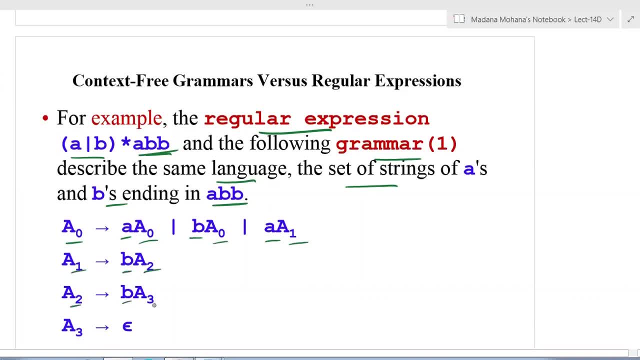 null. so whenever you can derive any string from this grammar, these strings can be derived from the language also. that is a plus b. cache closed: ab. you can derive any string from this grammar. that string must, judging that effect is going to be of course, hear and b b in here. uh, you can. 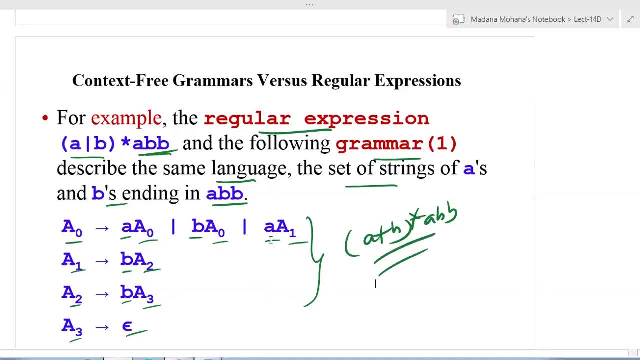 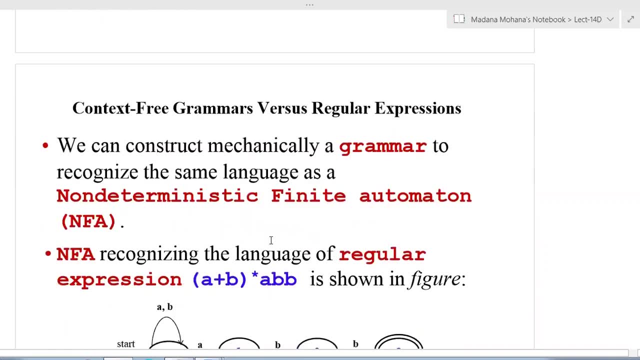 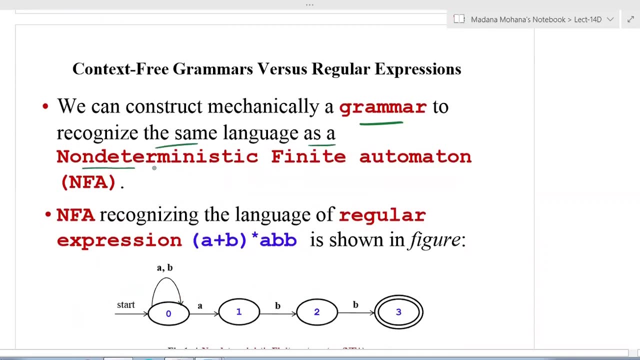 belongs to this long ways. So like that we can establish regular expressions and grammars relationship. So now here we can construct mechanically a grammar to recognize the same long ways as non-deterministic finite automator. So now, from the grammar we can construct its. 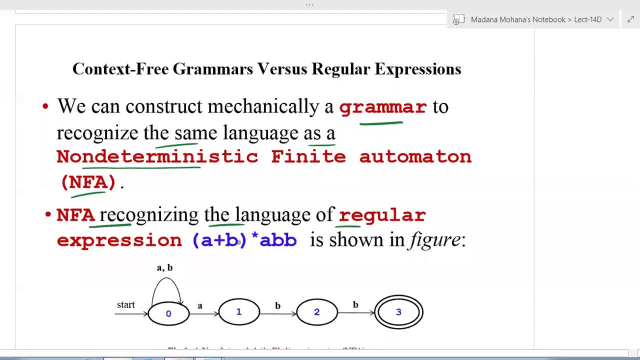 non-deterministic finite automator. And if we recognize the long ways for regular expression a plus b, whole closure a b, b, So the automaton for regular expression 2: you can construct NFA with epsilon or NFA without epsilon. This concept we discussed in our previous unit. 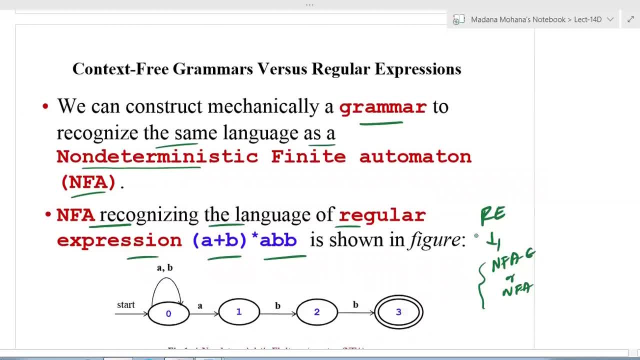 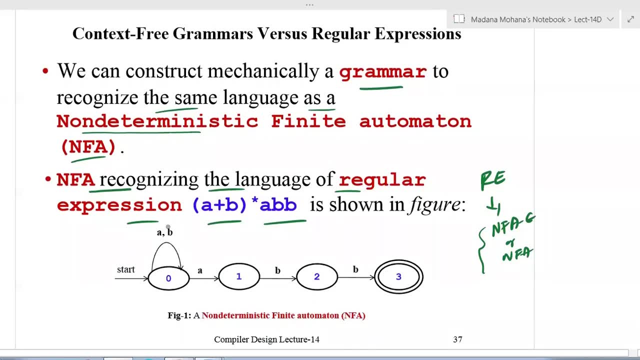 So many examples also. we demonstrated Now this is a direct NFA without epsilon moves is constructed here. Now, if you can combine all the interrelationships of the input symbols again, you will get the same regular expression. Now you can see a, comma, b loop. 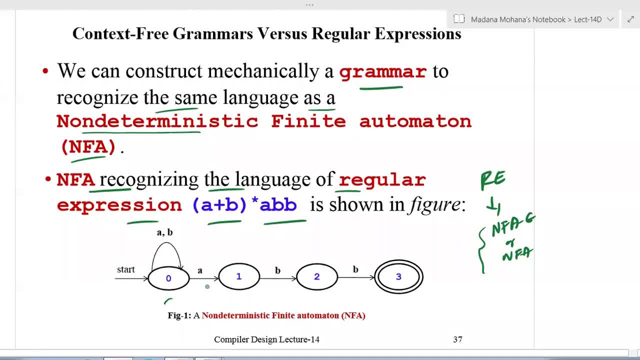 means this is nothing, but this is a plus b, whole closure. Now this is concatenation a, again concatenation with b, again concatenation with b. Now you can see a plus b, whole closure. a b, b, Our required regular expression is derived. Now this is the NFA. This is not DFA. Why? because 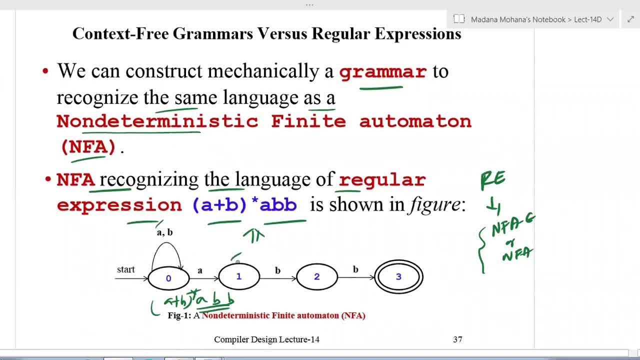 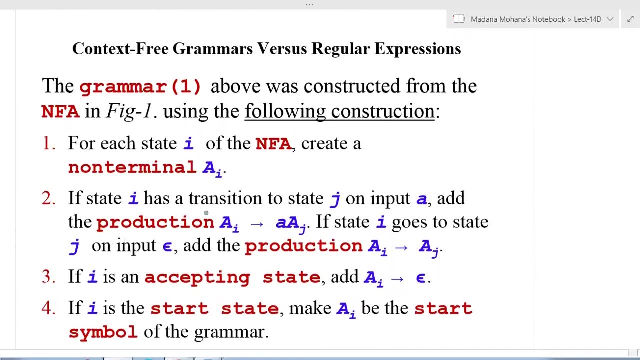 from state 0 on a. we have two transitions: one is 0, one is on 1.. So this is NFA. Now, from regular expression 2, we will construct NFA for recognizing the regular expression. Same for will apply for grammar also. From grammar also, we will construct the automaton. The following: 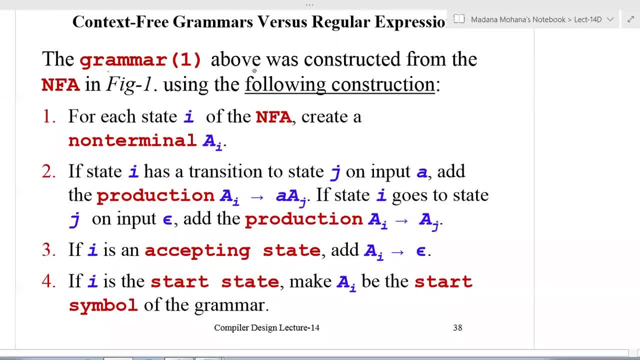 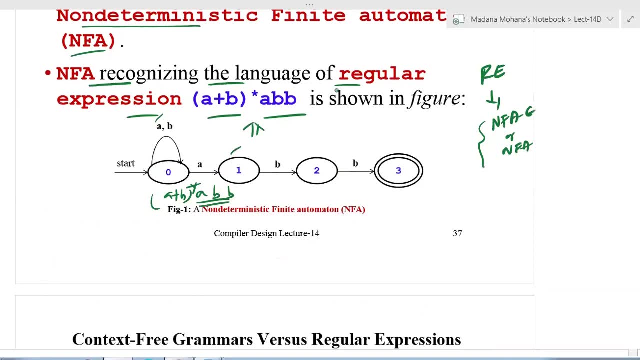 procedure is used. So the grammar, the above grammar, was constructed from the NFA in figure 1 using the following construction: So once we know the NFA using NFA directly, we can construct its grammar also, Then grammar to automaton also Here both conversions. 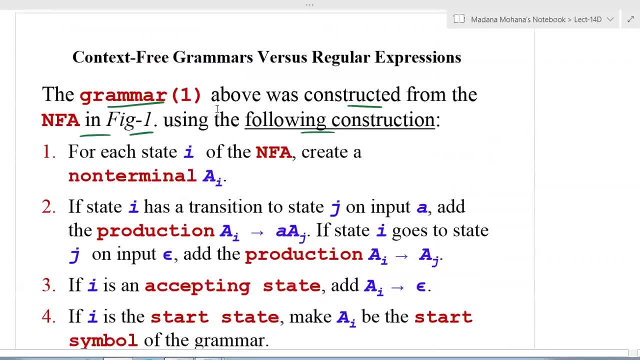 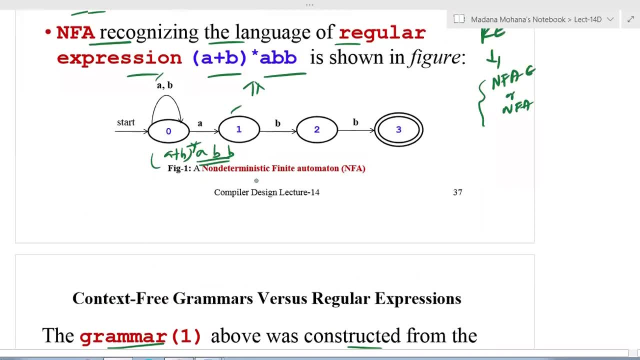 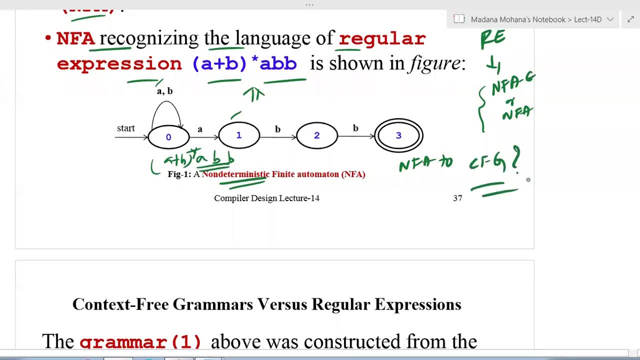 are possible. So now here what we are doing: the grammar one. the above grammar was constructed from the NFA shown in the previous. This is the NFA, From this, now NFA to context free grammar. How to construct? So by using the following procedure, Now for each state i: i is the state i. 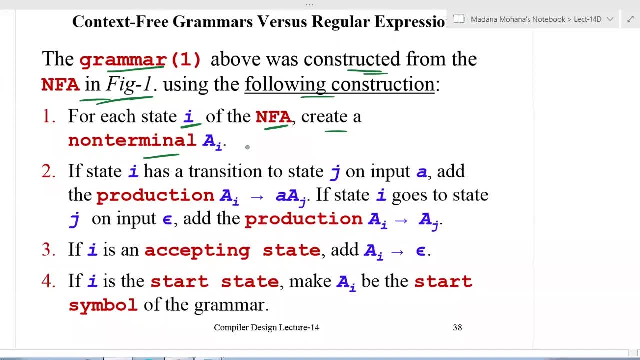 of the NFA, create a non-terminal ai For every state i. you can make it as a non-terminal with a subfix, Capital A, a subfix. So now, for example, here i equal to previous one, 0, 1, 2, 3.. Now here a, 0, a, 1,, a2, a3.. These are all the variables of the context free. 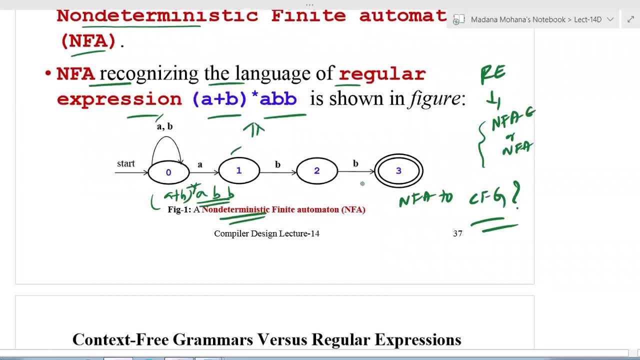 grammar Now you can see 0, 1, 2, 3.. Now a 0 in non-terminal is no mental variable. Then we now now a naught a 1, a 2, a 3. these are all the variables of the context. free grammar now for. 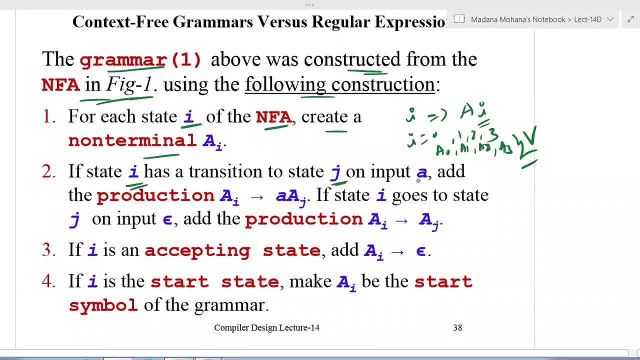 each state i as a transition to state j on some input a. then we have to add the production like this: a i derives the input a, then the next state is a j. now, here you can see: a i. this is nothing but state i. now. this is nothing but input symbol. now, this is nothing but state k. now you can write. 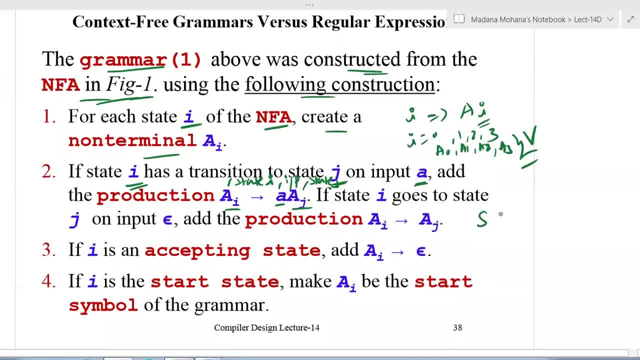 the corresponding production like this: that means delta of delta of 0 on input a. it is going to 1. let us- this is the transition, now the corresponding production: for this, the variable is 0. for this, the variable is 1. now you can write the production like this: 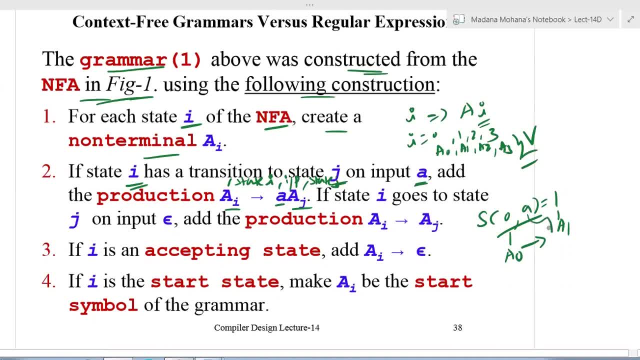 a 0 derives, then the input symbol goes to the right hand side, leftmost now a. so this is the production from transition. you can write the production like this: then, if state i goes to state j with input as epsilon, then you can add the production without input in the right hand. 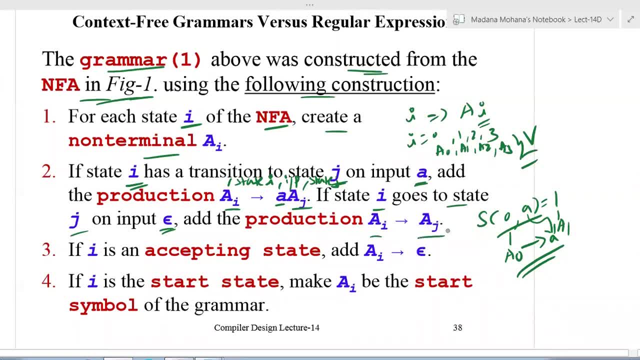 leftmost. now, simply, you can take a i derives a j, a i derives a j. here this is null actually, so you can't include null by default. empty means null only so if any state going to any other state with nfa, with epsilon, then you can write the production with the left hand side. 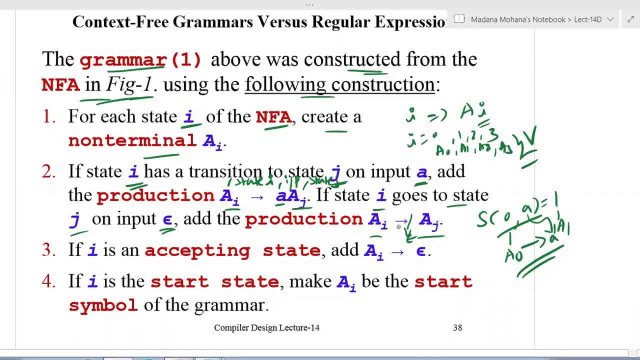 state derives. right hand side with respect to variables: here no input symbol is included. then the third rule: if i is an accepting state, then you have to add a null production starting with the variable a. i, a, i derives null. then if i is the start state and make a i be the. 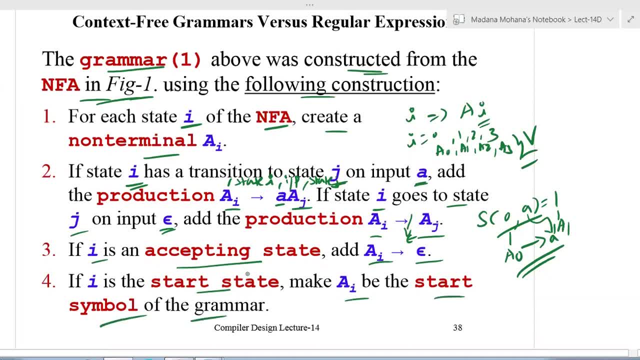 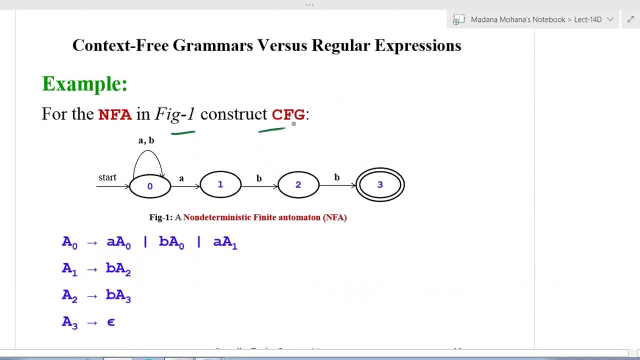 start symbol of the grammar. so these are all the four rules which are used to construct a context free grammar for the given nfa, even with or without epsilon. also. now the same example, let us see here now for the nfa shown below: construct context free grammar. so now here the states. 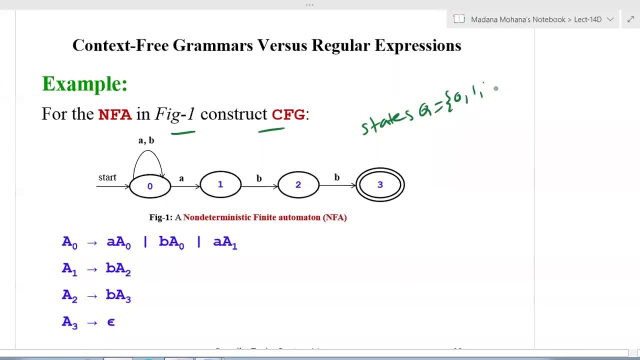 states capital q equal to zero, comma one, comma two, comma three. now you can convert into where variables as: v equal to a naught, a1, a2, a3. now these are all the variables, now the starting variable by default. first one here s equal to a naught starting variable. so now the productions. 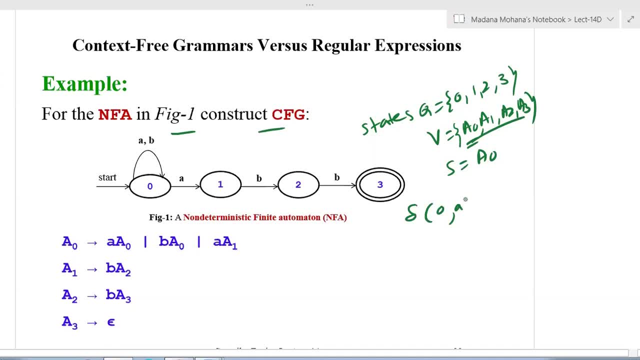 first you can see the transition. delta of 0 on a equal to this is going to 0, comma 1 for this now the transition. you can write like this: first for this: a naught derives, a, a naught one, but one at a time you can take. then again: a naught derives. 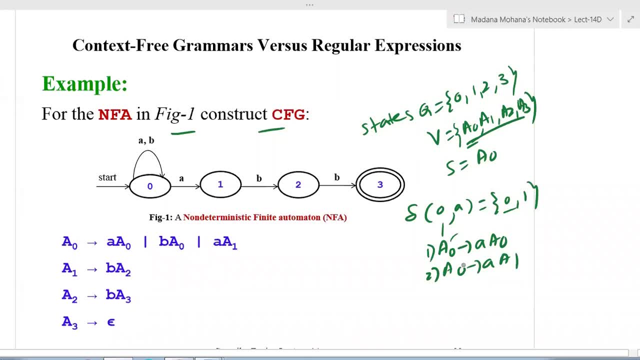 a, a1. so these are all the two productions starting with a naught. so then for zero state. on b also, we have other transition: going to zero, going to zero state. so now this can be for this: the production is a naught, derives b a naught. 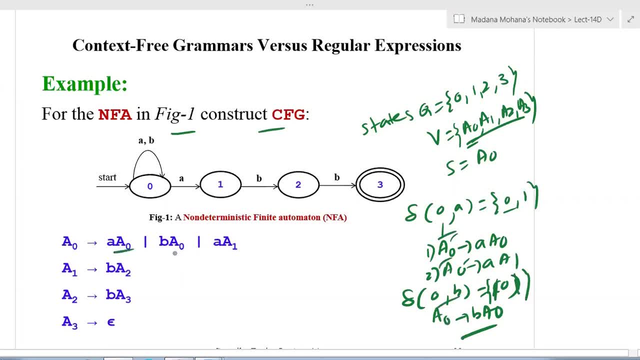 now all the production, starting with a naught. you can combine a a naught or b a naught or a a1. so now for a state one, delta of one on b equal to two, it is going to state two. now for this: a1 derives b a2, so this is the a1 production. then from state two, that means a2. so 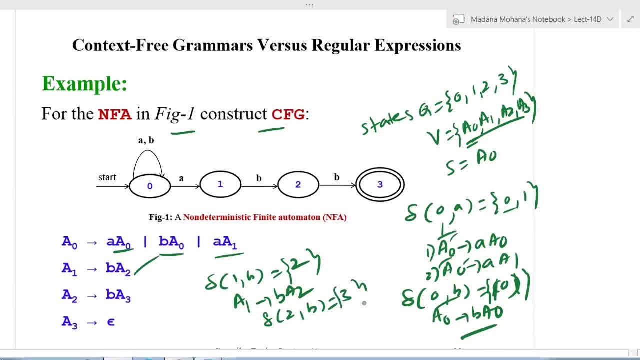 delta of two on b, it is going to state three derives BA3.. Now this is the A2 production. Now for final state. here A3 is the final state. you can add a null production. Therefore A3 derives null. So like this, using the: 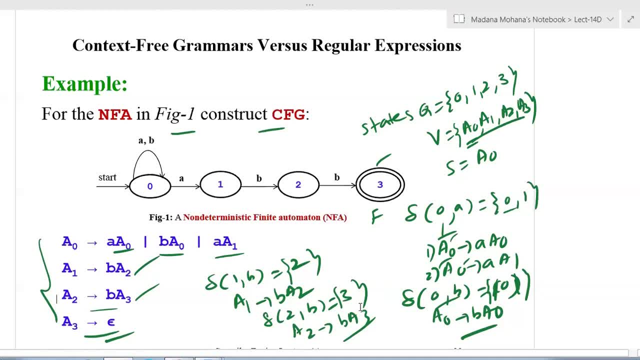 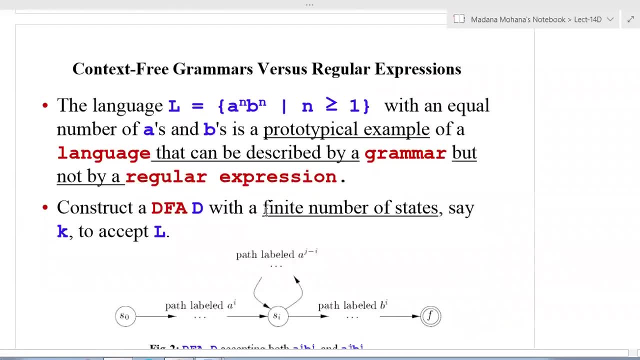 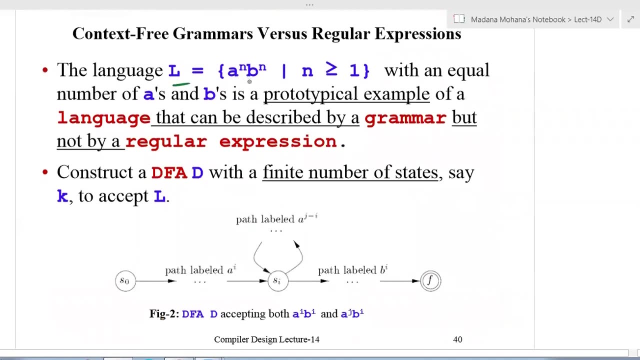 above four rules, you can construct a context-free grammar from the given finite automaton. Now let us continue with the other variations. Suppose a language L equal to A power and B power such that N greater than or equal to 1 with an equal number of A's and B's. 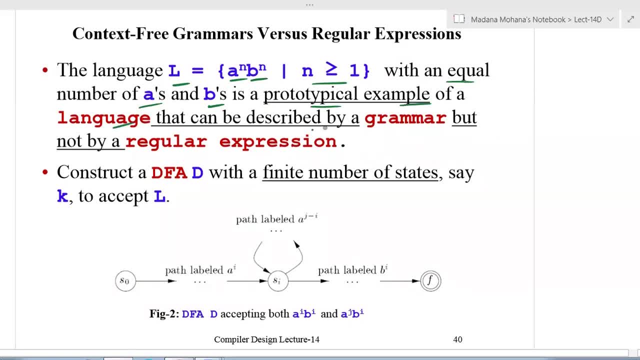 is a prototypical example of a language that can be described by a grammar but not by a regular expression. So here construct a DFA D with a finite number of states, say K, to accept the language L. Now this is the skeletal DFA for this language: A power and B power such that N greater than 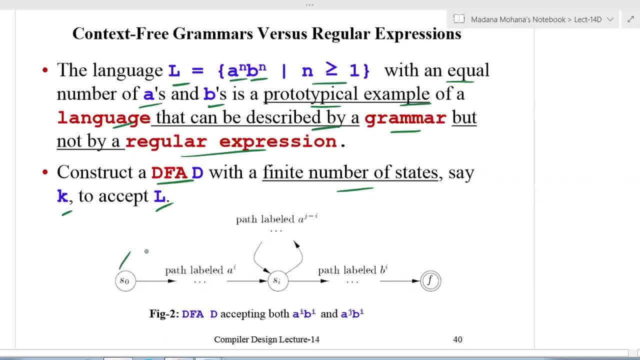 or equal to 1.. Here our starting state is S- naught, then path labeled with A power i. then next state is S- i, here labeled with A j minus i. then next state is F, which is final state, path labeled with B power i. Why? Because here this is infinite language. 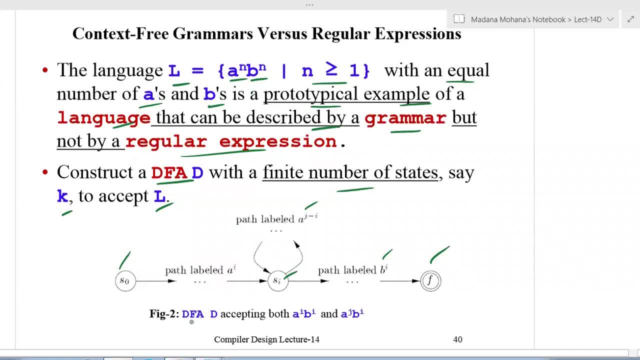 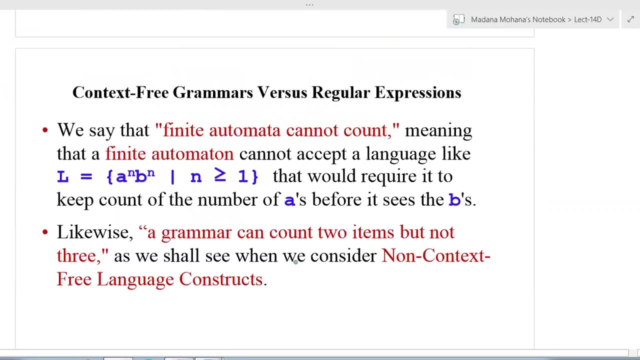 so general DFA is shown here. So the figure shows DFA D accepting both A power i, B power i and A power j B power i. So this is the one sample DFA for the infinite language. Now, with this, let us see some observations. 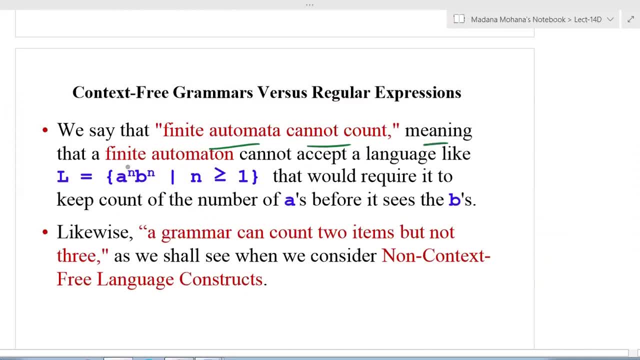 We say that finite automaton cannot count, meaning that a finite automaton cannot accept the language like A power and B power, such that N greater than or equal to 1. That would require it to keep count of the number of A's before it's its number of A's. So 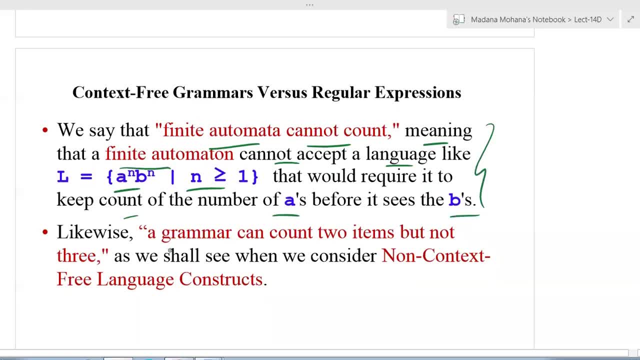 this is the reason Then, likewise, a grammar can count two items but not three. A grammar minimum will count two items only, as we shall see when we consider non-context-free language constructs later upcoming topics. Okay, now let us come to the summary of this lecture. 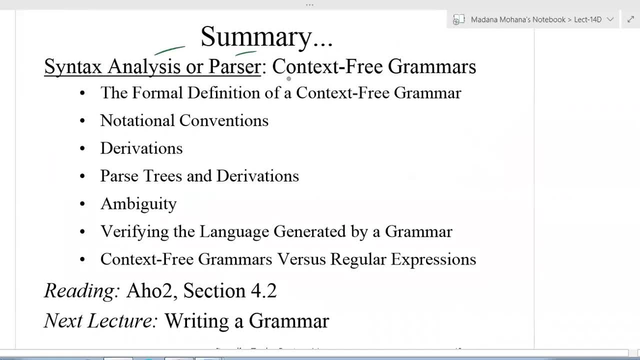 what we discussed As part of syntax analysis or parser, we discussed the context-free grammar amentation Under CFG. first we discussed formal definition of CFG and rotational conventions, then derivations – various types of derivations with examples. Then pars drives on derivations. 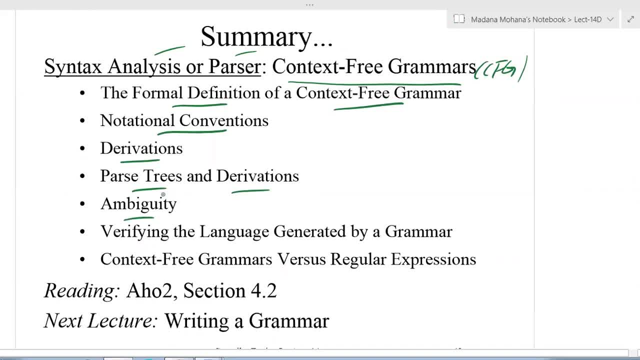 then with example, then ambiguity definition with example, then verifying the language generated by a grammar, then context-free grammar versus regular expression. For this lecture, the references is how to section 4.2.. Next class we will come up with other. 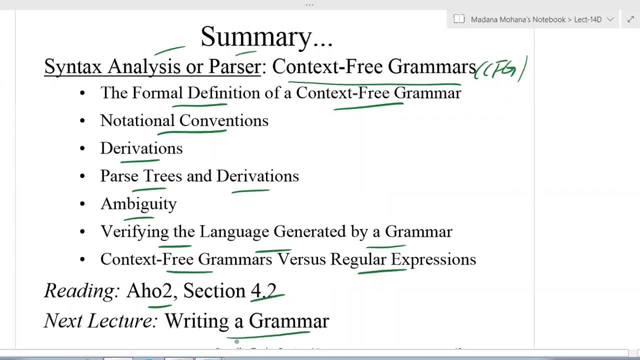 new topic related to this context-free grammar. Thank you, context free grammar- writing a grammar. So here we will discuss about how to eliminate ambiguity, followed by some other transformations on grammar. Now I stop here.